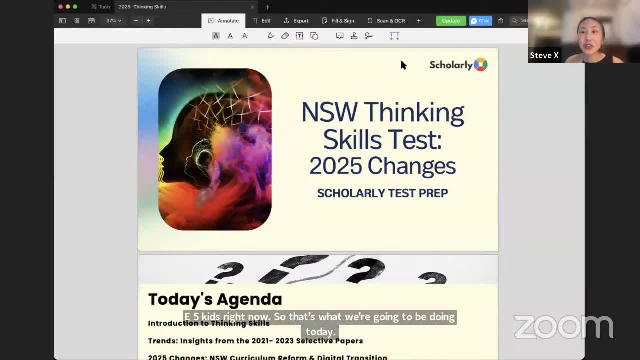 what we're going to be doing today, And I hope that you guys find this useful. I hope I bring some clarity into what's going on, because unfortunately, there's not a lot of information out there. So what I've done is I've tried to gather all the information I could get. 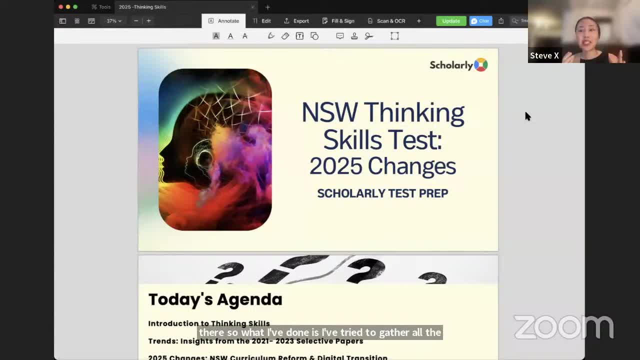 and I've tried to kind of come up with my best advice for the year five kids doing the new format thinking skills test. Now not much has changed, so rest assured I don't want anyone to stress but there has been a few kind of changes in the interface and some changes in the New South Wales. 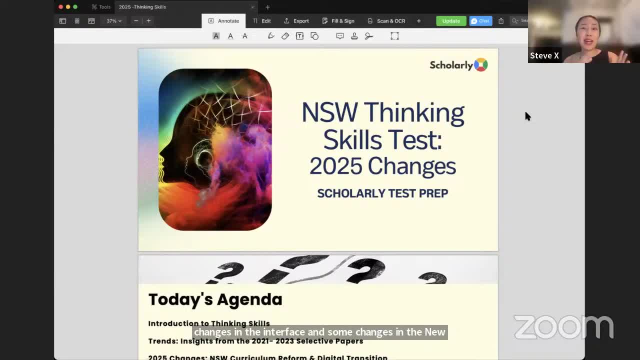 curriculum, which I'll also discuss. So I'm going to talk about how that might impact thinking skills. Before we begin, let me just introduce myself. So my name is Jen. I am one of the first tutors ever here at Scholarly. I've been 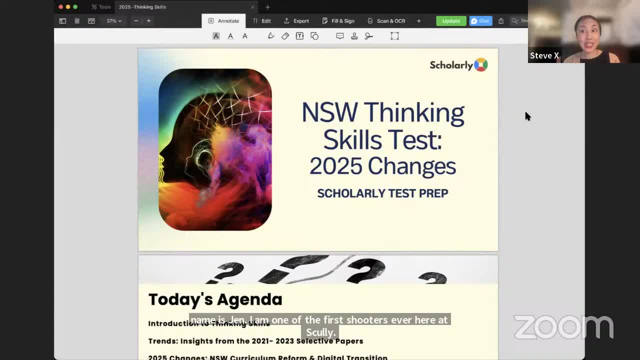 with Scholarly since its inception and I've really seen it evolve throughout the years. I've seen the transition from GA to thinking skills and we've adapted to that transition, although it was a huge, huge change, And I'm very, very proud of all the results that our students have achieved over the 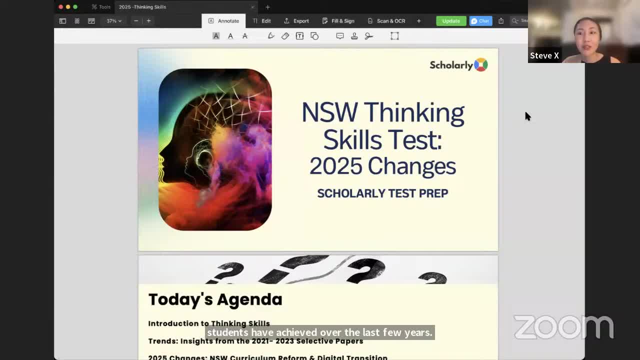 last few years. So I'm going to talk a little bit about what's going on in the New South Wales. I hope that you guys- everyone in year five or year four, if you're watching- can continue this trajectory of success. I know you guys can do well, so let's get right into it and let's talk. 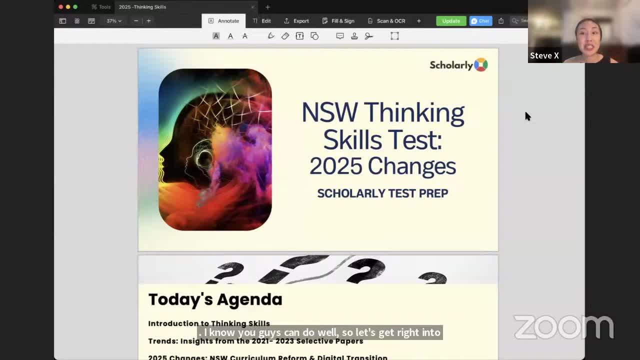 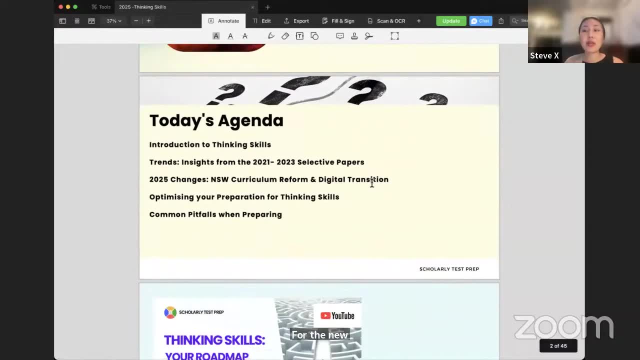 about what we can do in order to adapt for the new 2025 test. Okay, so today's agenda. what are we going to be talking about today? We're going to be quickly discussing thinking skills and the various trends in the past few years. So the insights that we have garnered from the 2021 to the 2023. 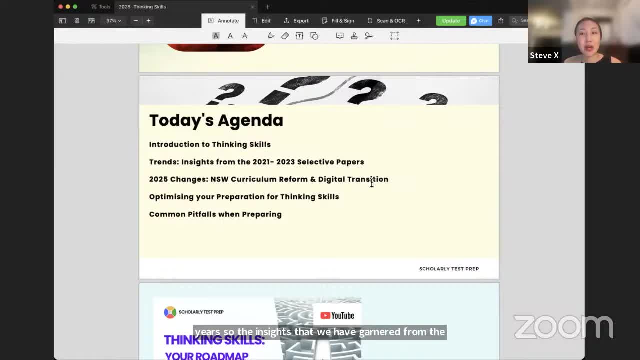 papers. Then you know what you guys have come here for. tonight I will be talking about the 2025 changes specifically to the New South Wales curriculum reform and how they've integrated critical thinking to all subjects and how that's going to affect thinking skills, And then I'll 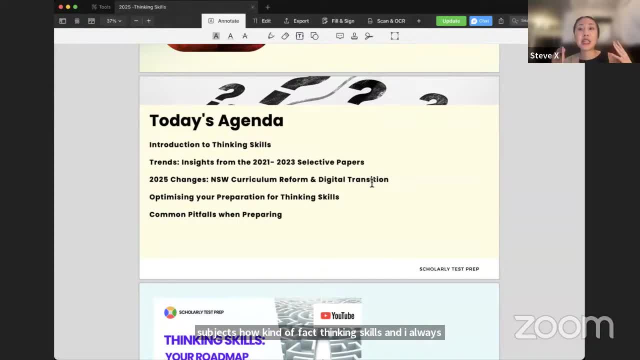 also be talking about how you can prepare for the computer-based test. So I'm going to be talking about how you can prepare for the computer-based test And then I'll also be talking about how you can prepare for the computer-based test. So I'm going to be talking about how you can prepare for. 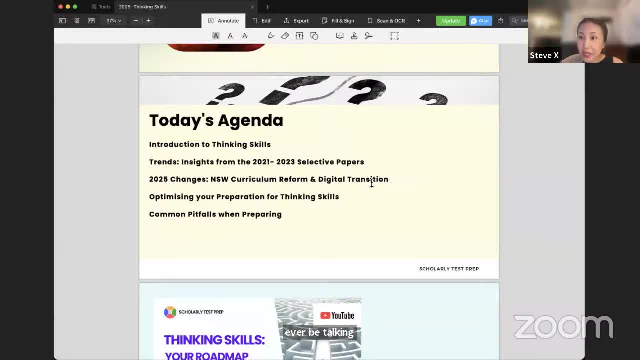 Now we'll talk about optimising your preparation for thinking skills. There's some secret tools that you can use that can really really help you. So I'll touch base on that And then I'll also quickly talk about common pitfalls when preparing. So I hope that you guys find this. 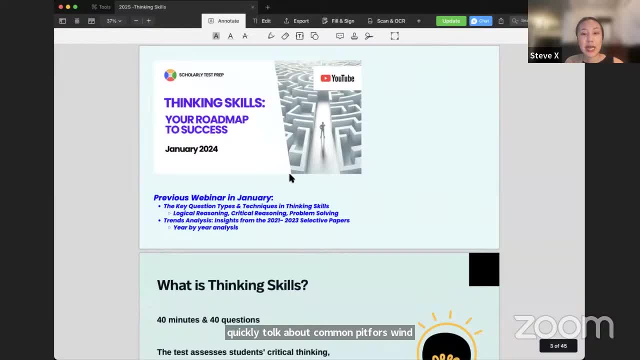 useful. Now just a quick kind of PSA. This webinar tonight is not meant to be teaching webinar, in that I'm not going to be, you know, going through questions. The goal today is for me to answer all of your questions, So I'm going to be talking about how you can prepare for the. 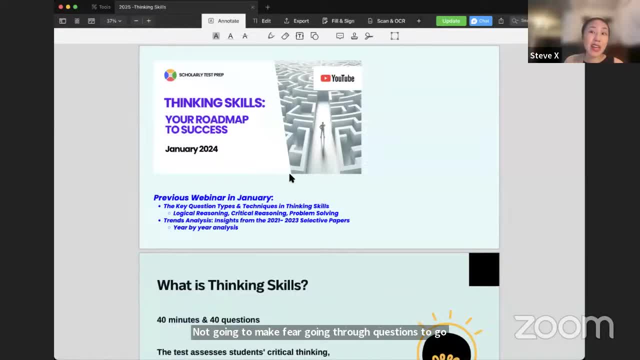 actually kind of give an overview of how you can independently prepare for the test and how you can go about maximizing your chance for success. based on the new someone's requesting for AI companion. can you please stop requesting, because that pop-up is always coming up, okay, anyway. so what I'm going? 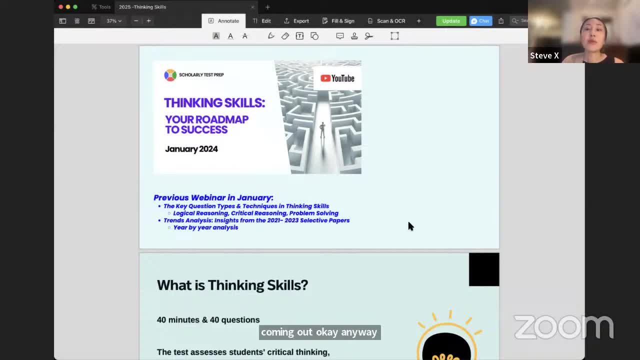 to do today is talk about changes and also how you can moderate your own study approach in order to do well. okay, so we're not going to be talking about specific question types. if you want a more kind of comprehensive breakdown of the question types, please go watch my January webinar, I think. 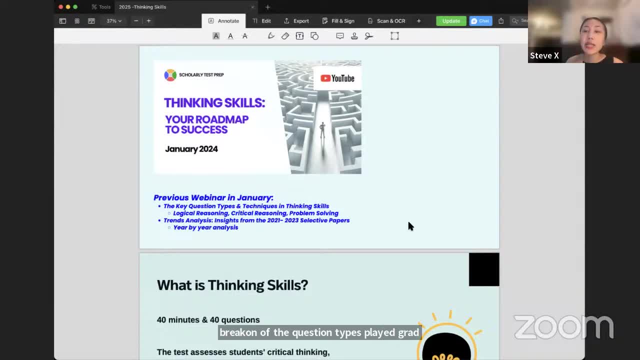 it will be on YouTube, so it's been recorded, and in that webinar I basically go through all the key question types, all the techniques and skills that you generally need in thinking skills. that's the goal of today. okay, so I just want to make it very clear. 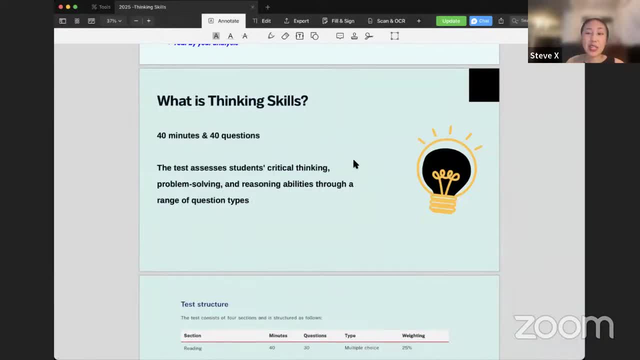 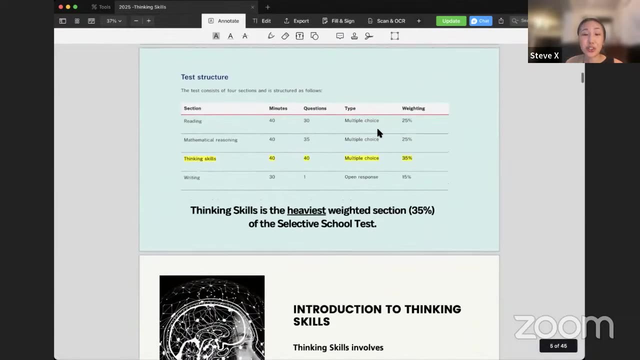 let's just quickly talk about thinking skills. I know you guys already know what it is, but it is a section in the selective school test: 40 minutes, 40 questions assessing critical reasoning, problem solving and logical reasoning. okay, now it is actually the heaviest weighted section of the 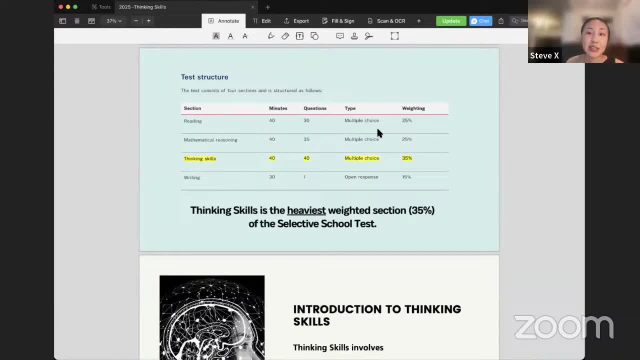 selective school test. it's weighted 35, which is quite significant. so the New South Wales DOE- they have scrapped school marks, so all of your marks are completely dependent on how you do on the day. and thinking skills is 35%, which is quite substantial compared to mathematical reasoning. 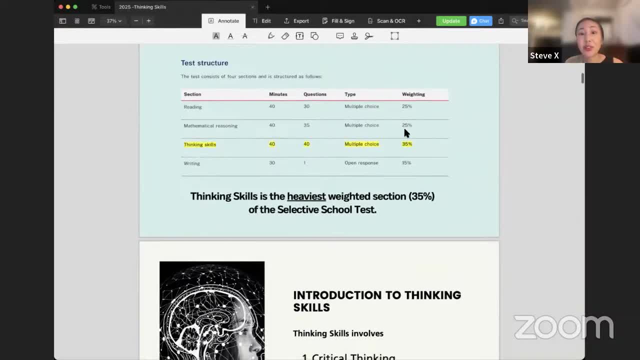 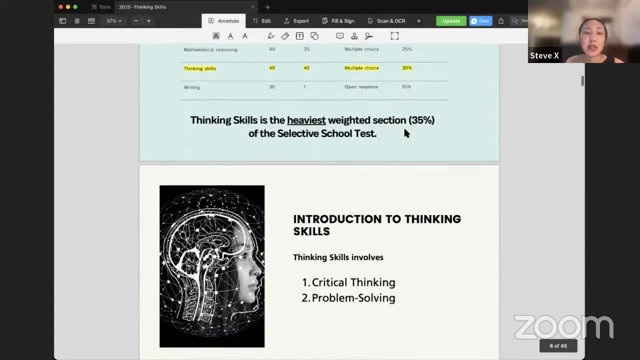 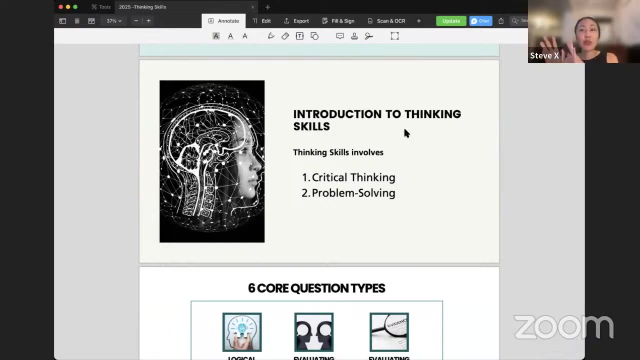 which is 25%, reading, which is 25% and writing, which is only 15%. so if you want to do well in the selective school test, doing well in thinking skills can really help, okay, um, now, broadly speaking, two main categories of question types. so there's critical thinking, which is all about argument. 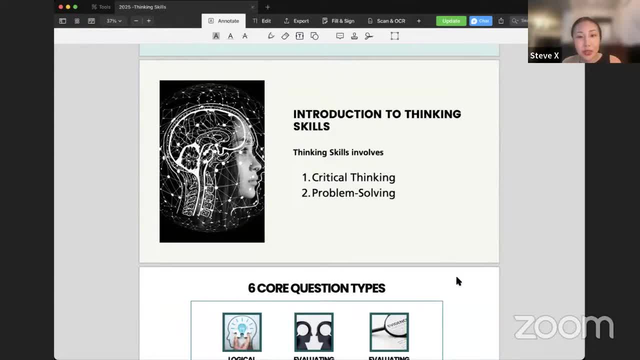 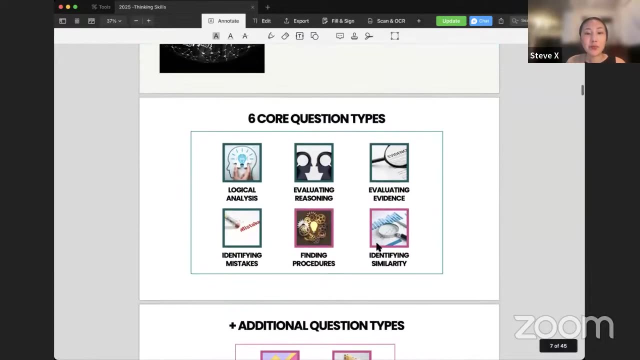 analysis, right, and problem solving, um, now there's a bit of overlap in these question types, so not all questions are clear cut. there's somewhere. there's a bit of both. but I'll be generally talking about these question types. then I'll talk about, you know, the juice. so, again, I've talked about this in my January webinar, but 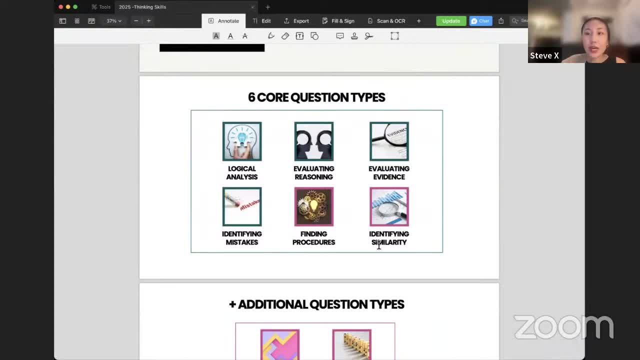 these are the six core question types that has been specified on the New South Wales syllabus, so you know they're pretty much giving away, like what you should be expecting. there's logical analysis. there's evaluating reasoning, evaluating evidence, identifying mistakes- all those in blue they're the critical reasoning type questions. then we have finding procedures. 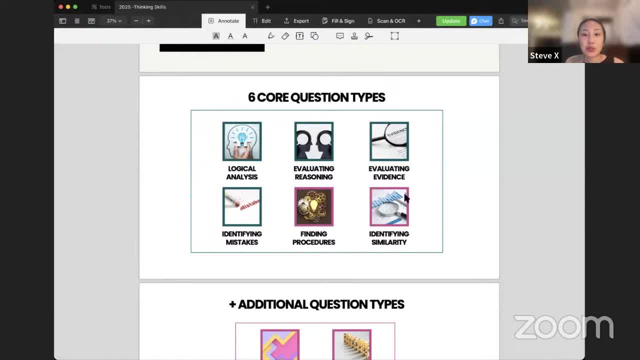 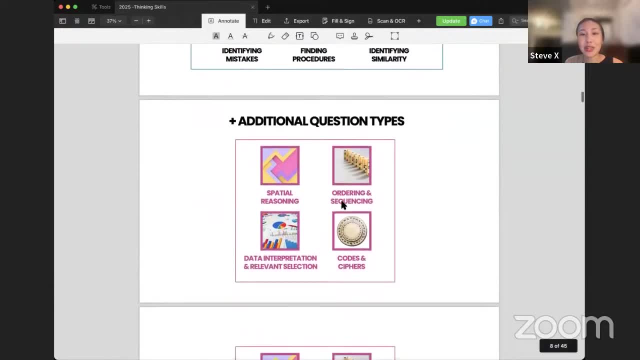 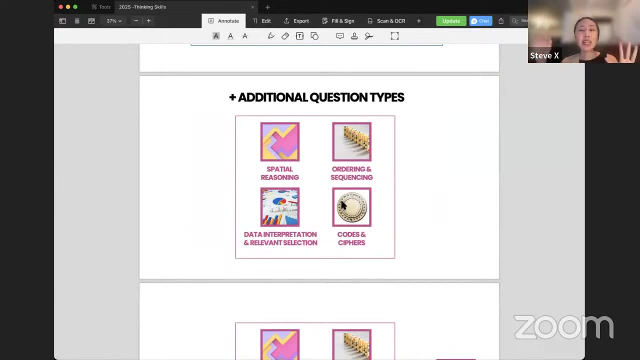 and identifying similarity, which is related to the data analysis questions. we also have finding procedures, which is very, very general, but it's what um they? this is the kind of question name they give to problem solving type questions. right, and that can encompass many, many different types. it could be spatial reasoning, where you have 2D, 3D shapes or maps. it could be ordering and sequencing. 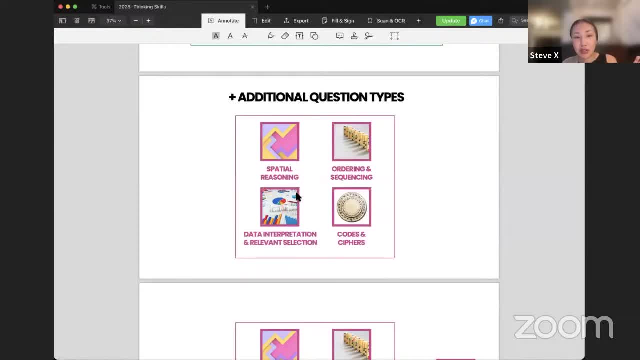 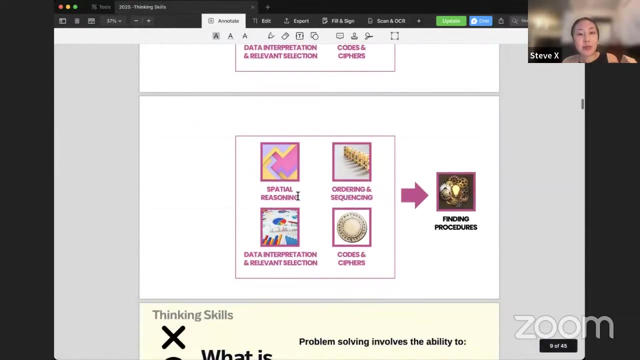 I love the ordering, sequencing games. um. it could be data interpretation, relevant selection, which is all about selecting relevant data from graphs, codes and ciphers. the list can go on, so it's very broad, diverse, unpredictable. okay, that's the truth. um. so these all fit under the umbrella of finding. 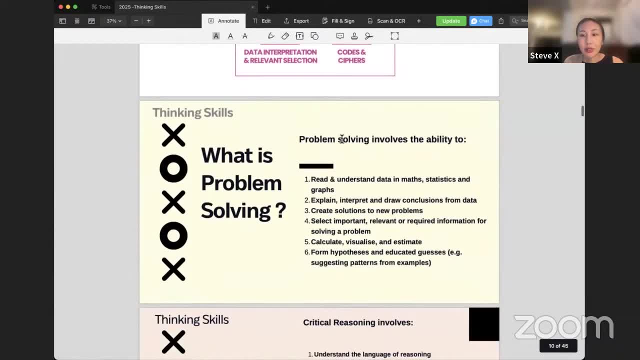 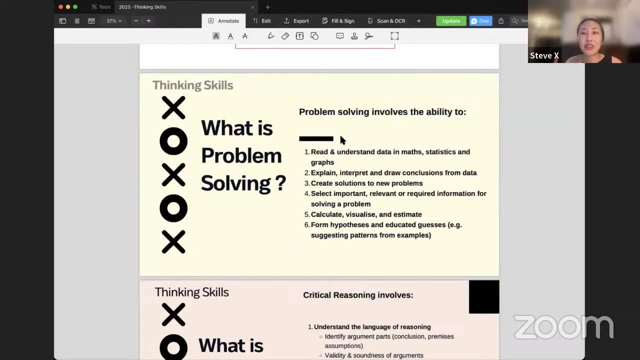 procedures. okay, now again I'm going to quickly touch base on problem solving. problem solving very general term. it's basically about solving problems, and that involves things like reading and understanding data and math, statistics, graphs, being able to, uh, fit together little pieces right, fill in the gaps. sometimes there's missing data, sometimes there's missing information, and your job is to 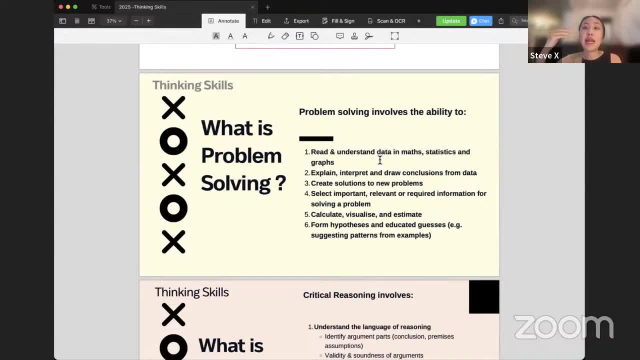 combine the information to come to a new conclusion, so to form a logical deduction from that information um to be able to explain, interpret and draw conclusions from data. to be able to create solutions to new problems, select important, relevant and required information for solving a problem, calculate, visualize and estimate, form hypotheses. 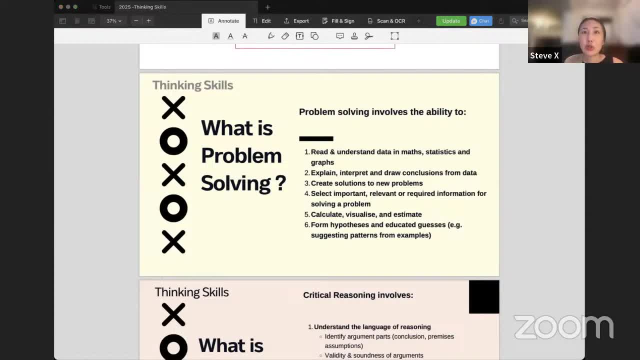 and educated guesses. now what does that mean? that just means that you have, um, you form a guess right based on the little information you're given and then you test that kind of like doing a science experiment right, but in a multiple choice question format. so that's an example of like the key skills. 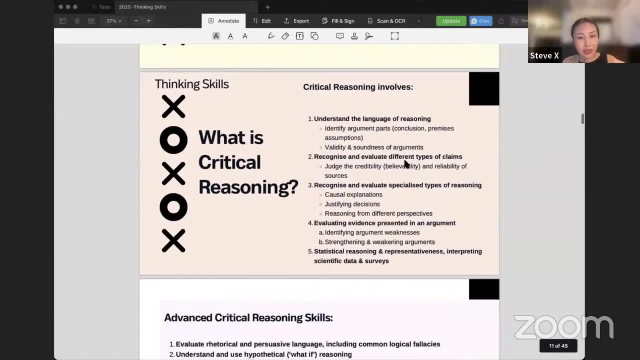 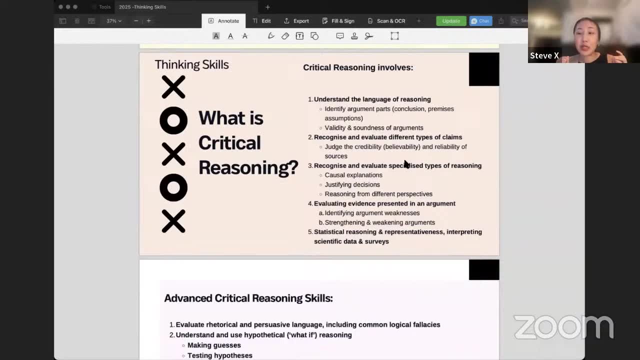 they're testing in problem solving. critical reasoning, on the other hand, is more about argument, so it's more about understanding the anatomy of an argument will really help. what I mean by that is understanding the parts of an argument- so conclusion, premises, assumptions, right- and then be able to understand the validity and soundness of arguments. so, again, this is stuff that we cover in. 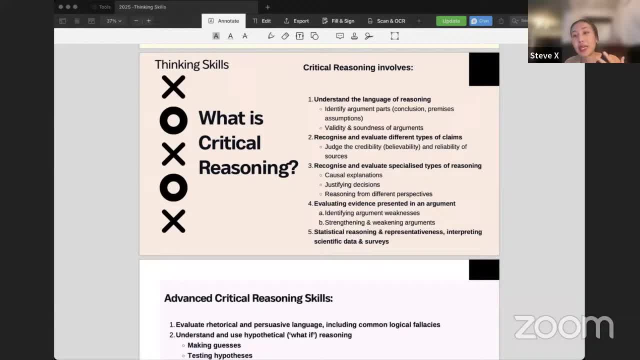 our lessons. but you might have heard of validity. validity is just when a conclusion logically follows from the premises. so if you accept the premises to be true, then the conclusion has to be true, right? and if that works, right, the argument makes sense, is valid. now I'm not going to be, you know, teaching you guys, because it's Sunday night, right, you guys? 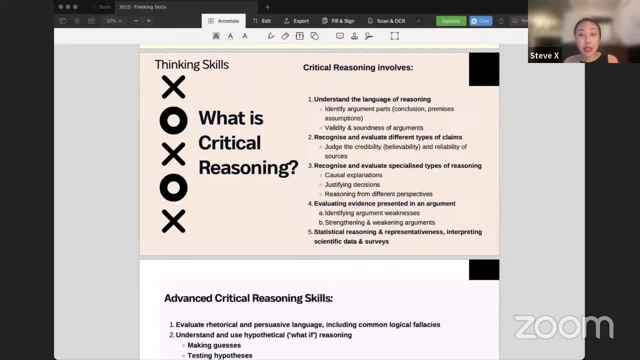 are on school holiday so I won't drag this out too long, but I'm just quickly outlining what you will expect in critical reasoning. uh, you might also be asked to recognize and evaluate different types of claims. so, understanding things like credibility, like how believable is that source, right there's. 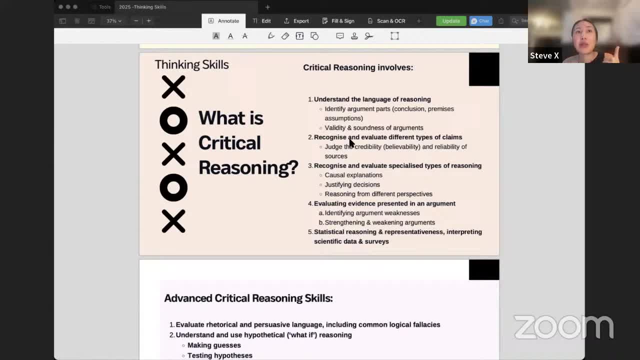 a lot of misinformation in the real world. there's a lot of distorted information and fake news. right, and if you're able to judge the credibility and the reliability of something, that is a very useful life skill, not just in thinking skills, but also just for you guys in the future, um be able to recognize and evaluate. 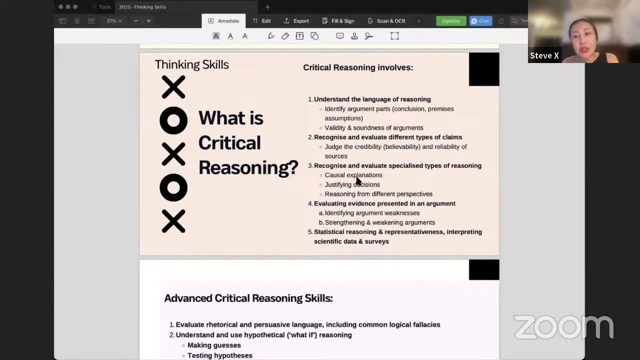 specialized types of reasoning. so there's causal explanations, decision making, justifying decisions, reasoning from different perspectives and then evaluating evidence. so that's just about being able to spot weaknesses in evidence, right? how strong is this evidence? does it actually provide good, solid support for the argument um and strengthening? 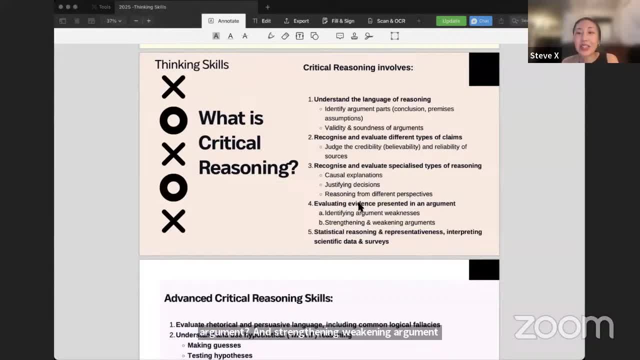 argument questions which you guys probably have seen many times in our practice papers. so, oh, and also they've started to introduce a few questions related to scientific data and surveys, and I think it's a very useful skill to be able to understand things like, uh, sampling bias, representativeness. 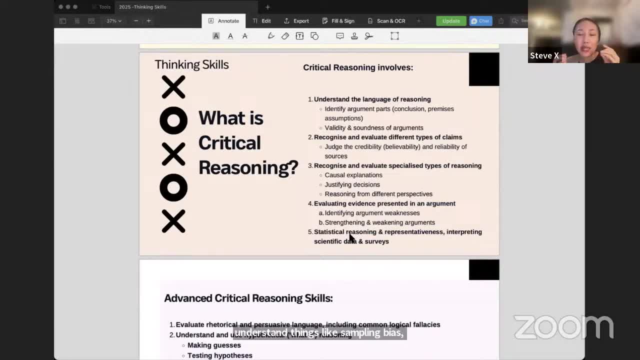 statistical reasoning and they're not like, obviously, in the syllabus, but they're the skills being tested like. you're given a question, maybe about a study that's been done and your job is to assess how well that study has been conducted. is it a well carried out study or is it poorly? 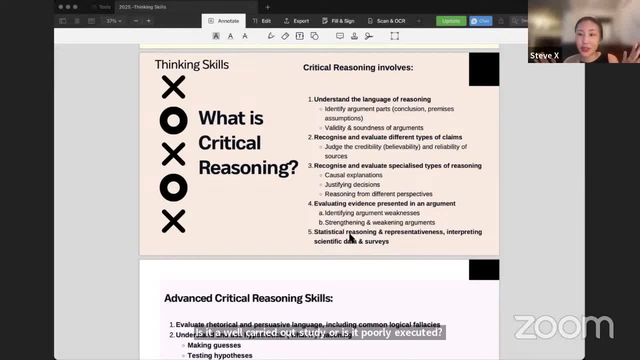 executed right and if you guys are interested in scientific research, that's a very, very kind of good intro into what you'll see when you get involved in research in the future. you have to conduct a well-designed study anyway. I'm just going on a tangent now, but there's some more skills and 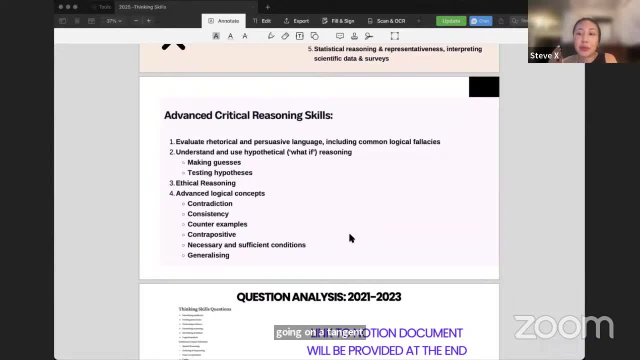 critical reasoning that, um, they are more advanced, but if you can develop them, then you'll do very well in thinking skills. themes include understanding rhetorical, persuasive language right understanding the ways that maybe advertisers or media might manipulate you. they might use certain appeal fallacies in order to 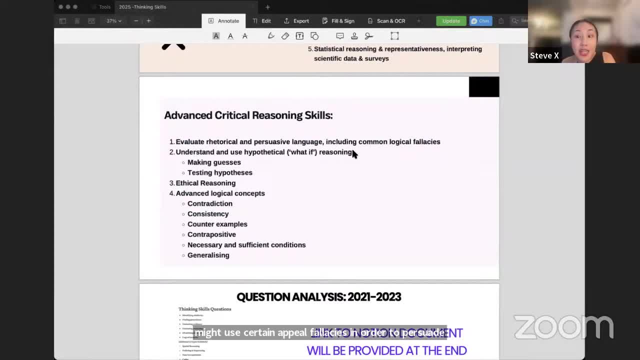 persuade you to do something right: understanding common logical fallacies. again, you don't need to learn any of them, but if you understand what they look like, you'll have a much easier time in the test, because they ask you find the mistake in the reasoning. you'll be like: yep, I know that's a. 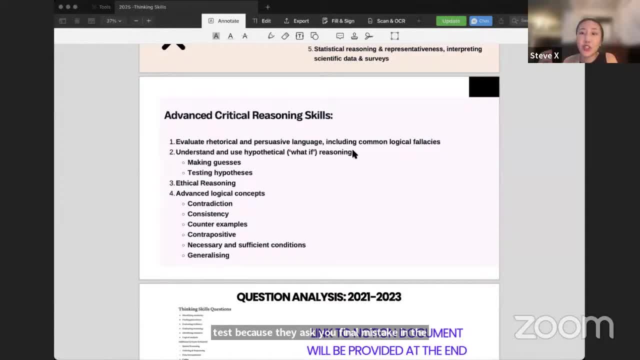 course fallacy- Well, I know that's confusing. a necessary and sufficient condition- Well, I know that's a straw man fallacy- things like that: Understanding and using hypothetical what-if reasoning, So being able to make educated guesses and be able to test these hypotheses. that will help you a lot. 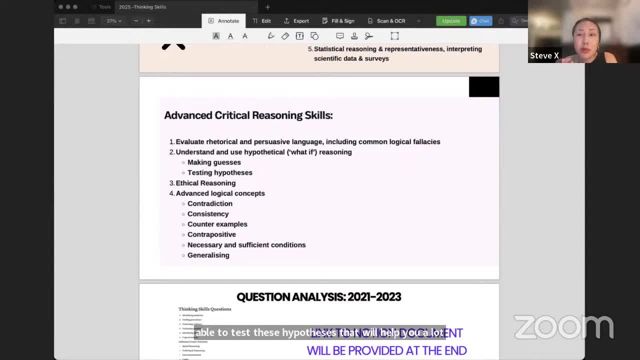 in the problem-solving questions as well, when you are able to spot patterns right And you don't have a clear-cut method. but what you do is you test different strategies right, Based on your intuition and based on gauging what you think is most appropriate, And then, if you've done very 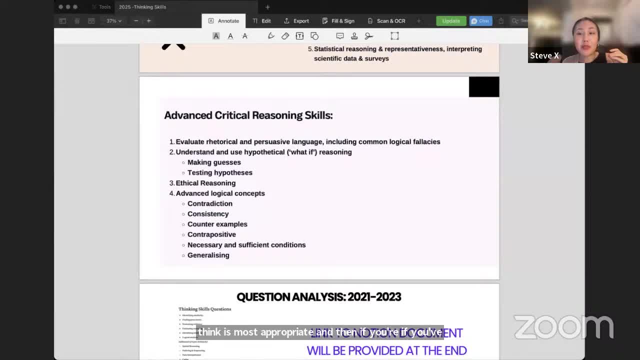 targeted practice, then you will be able to find the correct strategy a lot quicker. right, You'll be able to test your hypotheses in a very strategic way and you'll do well, because you'll get the question correct quickly And there's some more advanced logical concepts which I would not worry. 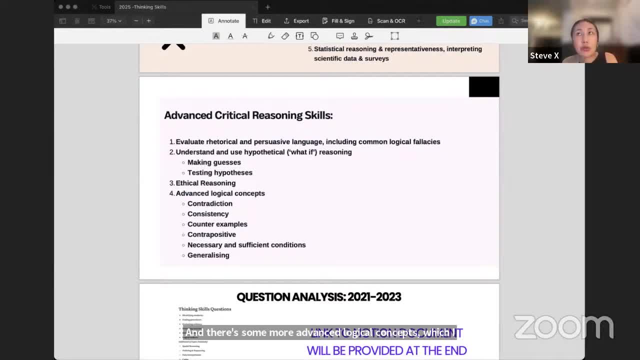 too much about, but there's things like ethical reasoning, So being able to assess what is right or wrong, or moral or immoral, Based on different frameworks. You guys are only five, so don't worry about that, But it's really interesting to study, like to understand how to approach ethical dilemmas. right, There's like a. 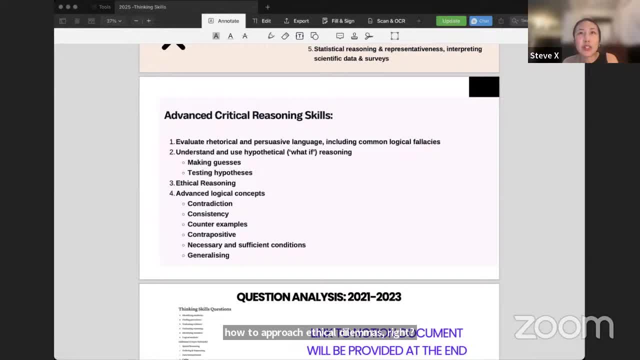 very oh, I can't even remember now, but there's like a very common question where, if there's like a train track going towards a certain number of people- like five people- and it's going to crash, like do you divert the train to kill the people on board Or do you keep the train towards the 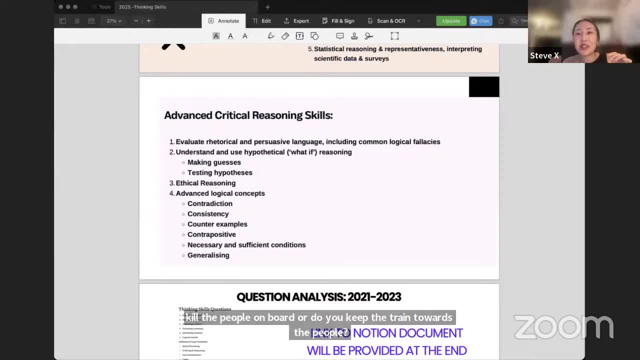 people. I can't exactly remember, I don't know what the specifics are, but to be able to answer a question like that, that requires some ethical thinking and it is challenging but very, very interesting. There's some other things, like advanced logical concepts, so contradiction, consistency, count examples. 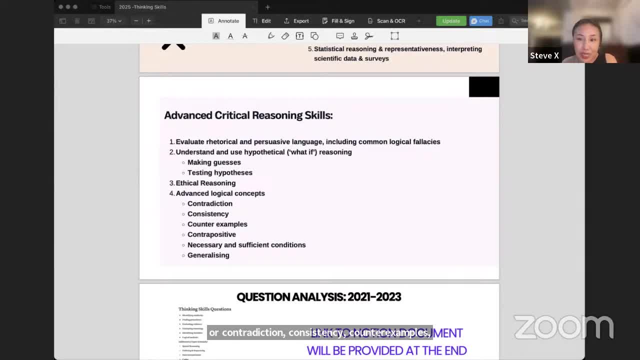 contrapositives, necessary and sufficient conditions and generalizing. Now, there's a lot right, And those are not skills that you need to study. Those are skills that you have to practice through questions, right? So that's a lot of things that you need to study And I think it's. 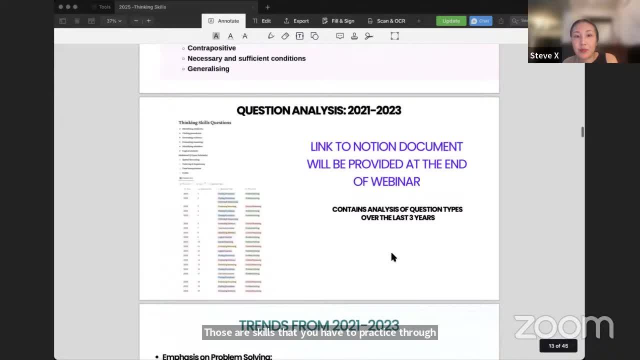 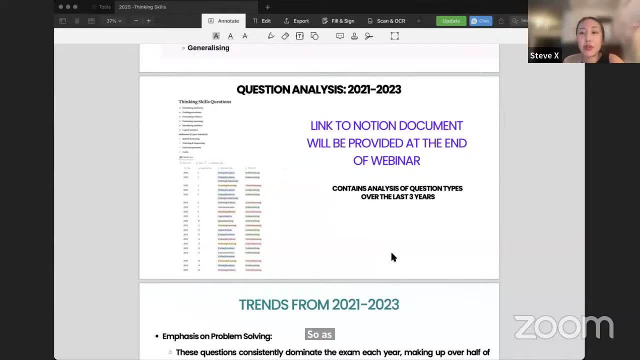 that's what I have to say about these critical reasoning skills. So, as I mentioned earlier in January, I've done a webinar where I did a more comprehensive breakdown of question types. I will try to make sure you guys have access to this Notion document because there 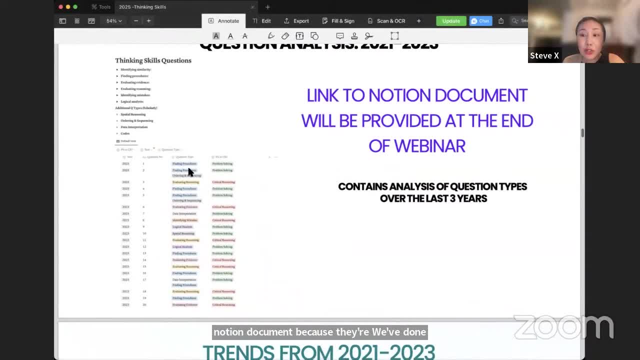 we've done a kind of question by question analysis So you can spot the overall trends. you can see, you know how frequent do we have those problem solving or finding procedure questions. How frequently do we have spatial reasoning questions? right And understanding that can. 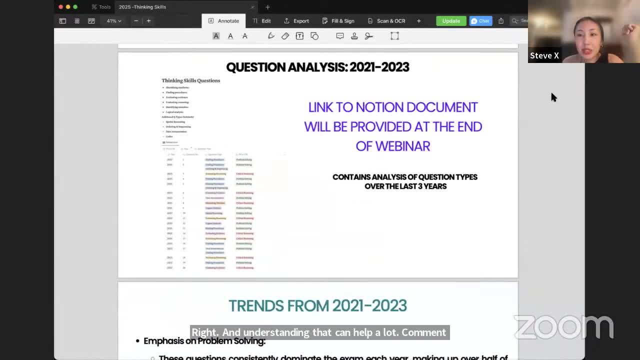 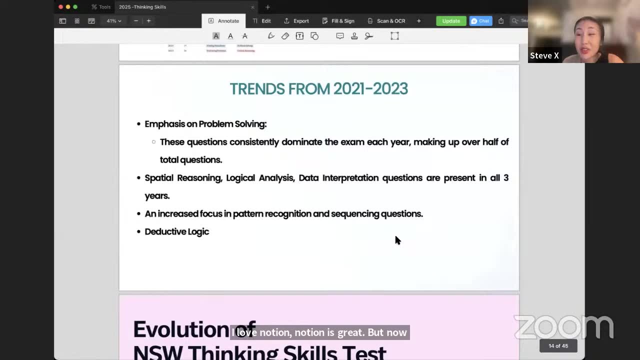 help a lot. Comment down below if you guys like Notion. I love Notion. Notion is great. Now again. I've talked about this in January, but the trends that we've seen over the last few years is that there's an increasing focus on problem solving. So that's what has happened. 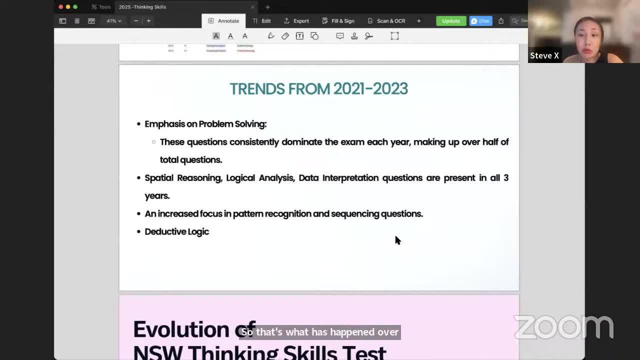 over the last three years. I can't say how the 2025 test will go or how this year's test will go, but there is a huge focus on pattern recognition and sequencing questions and deductive logic, which is basically questions involving formal logic, So questions where you are asked which of the following is true or not true. 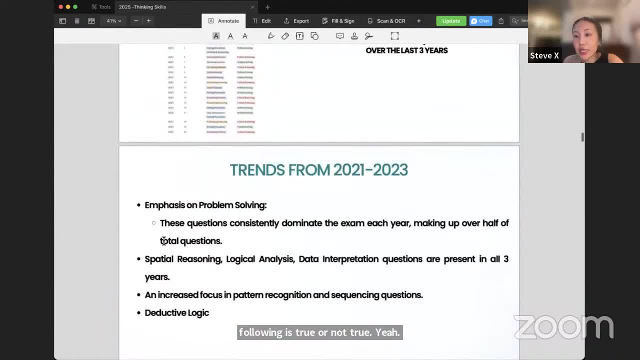 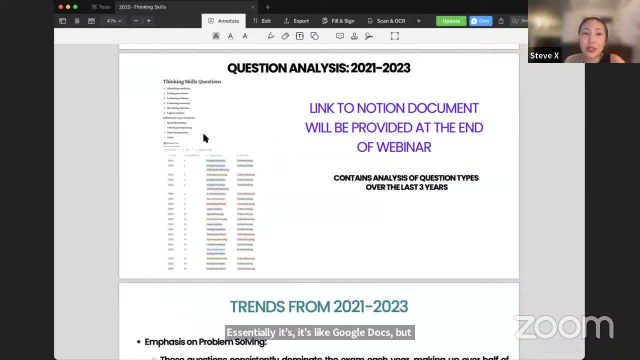 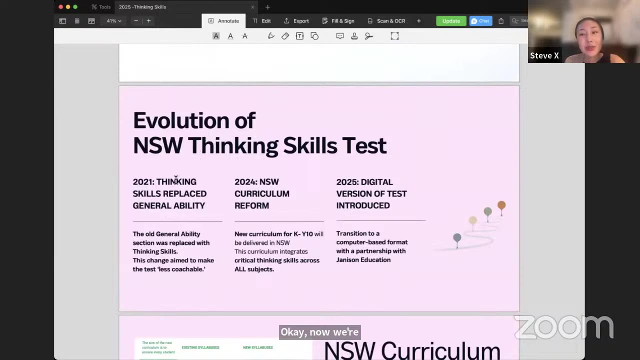 Yeah, Okay, And Notion is a note-taking app. Essentially, it's like Google Docs, but better, much better than Google Docs, in my opinion. Okay, Now we're going to talk about the changes of thinking skills throughout the years. So in 2021,. 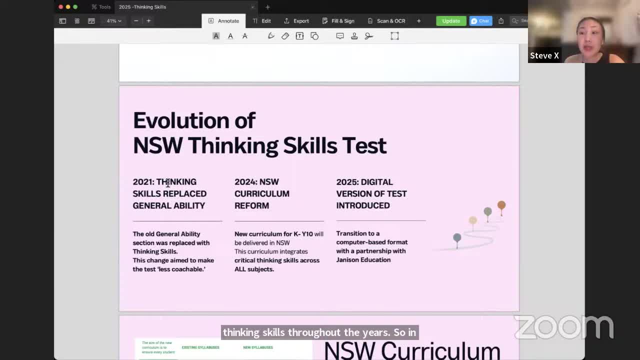 thinking skills was newly introduced. It replaced the old GA test And it's a lot harder than GA. So you guys, you're suffering because GA is a lot easier than thinking skills. in my opinion, Then in 2024, the New South Wales Department of Education has basically made a huge overhaul of the old curriculum. 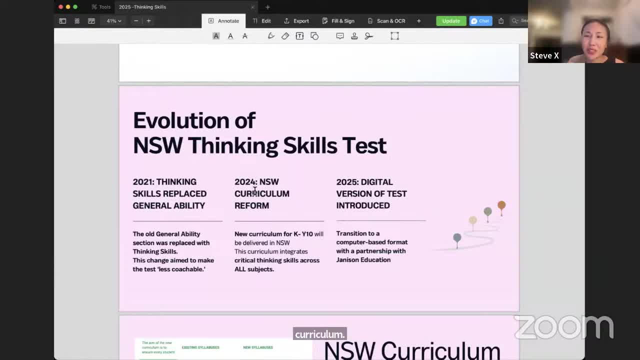 So curriculum is like a set of, like a syllabus that schools follow to teach kids. right, It's just like a document and schools look at the document and they're like, yep, this is what we should teach our kids. There's like a huge overhaul And now they really emphasize words like critical. 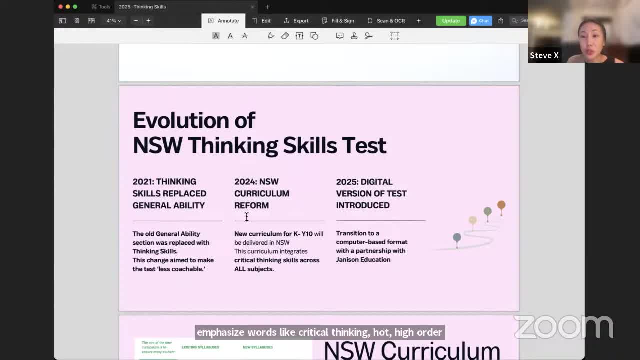 thinking, HOTS, high order thinking skills, which I'll talk about. right, You might be thinking: what on earth do they mean by that, Like what's HOTS, What's critical thinking? Again, it's all very general, but I'll try my best to explain what is going on. 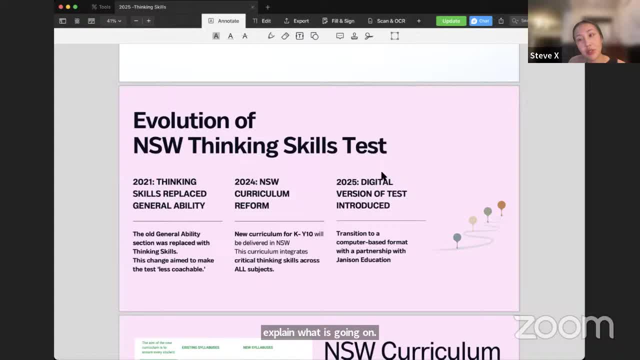 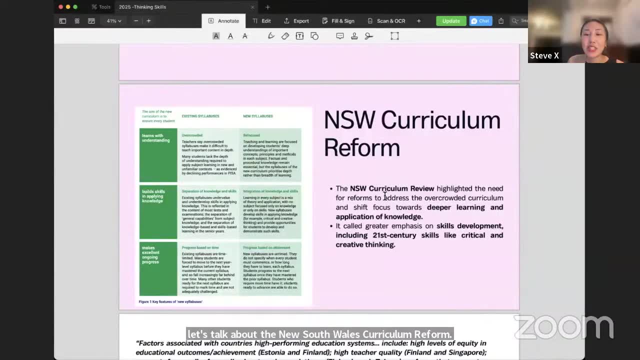 And then 2025, the test will be computer based. Okay, So let's talk about the New South Wales curriculum reform. Basically, they've essentially said: the old syllabus is not good because Australian students do the pizza test. It's like a test which assesses your academic skills. that 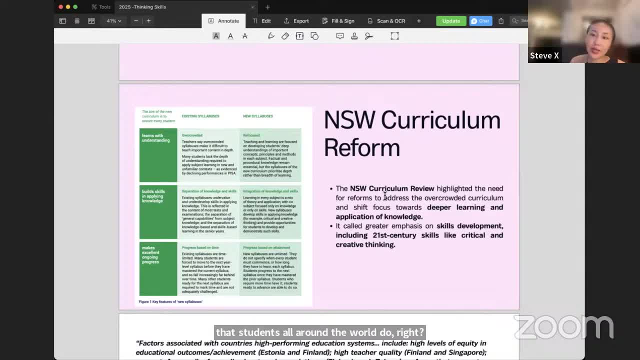 students all around the world do right, Like in China and Korea and Japan and Europe, like Italy, France, they all do that. Now, unfortunately, Australia has kind of not been doing so well, Like our performance has gone down over the last. 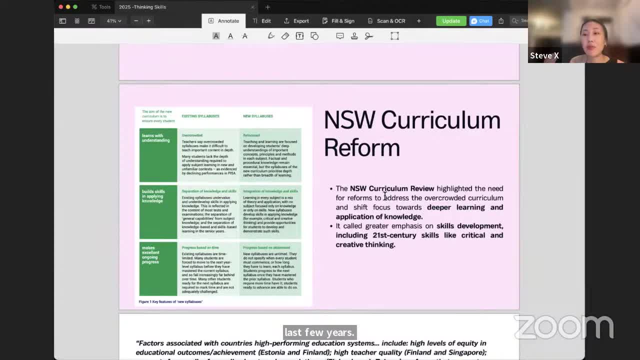 few years. So, as a result, they've like the New South Wales Department of Education. they're like we need to change, like we need to change something because we're going to change the curriculum. And now they're focusing on deeper learning and application of knowledge. Okay So. 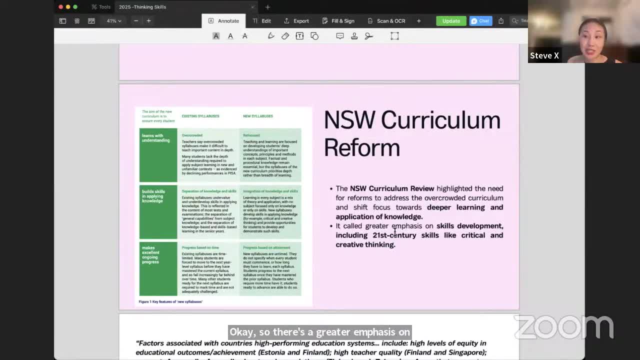 there's a greater emphasis on skills development, which sounds amazing, right. Skills development, including 21st century skills like critical and creative thinking. Okay, So they've gave like a very beautiful table on their curriculum. existing syllabuses- not good. new syllabus: better- Okay, And what are the key changes? Well, 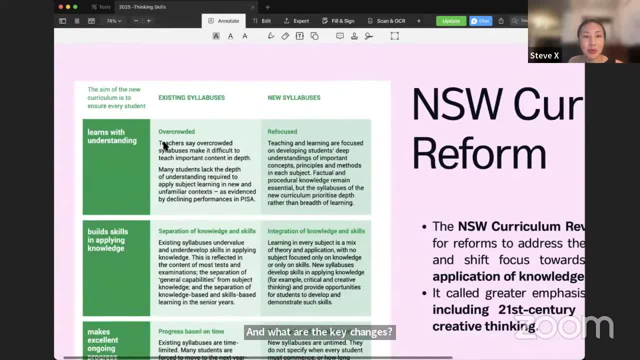 let's just kind of zoom in. It says before: overcrowded, difficult to teach important content in depth. So apparently maybe it was like there was too much information but not a lot of depth, So a lot of rote learning. I'm assuming that's what they're trying to say. And now they 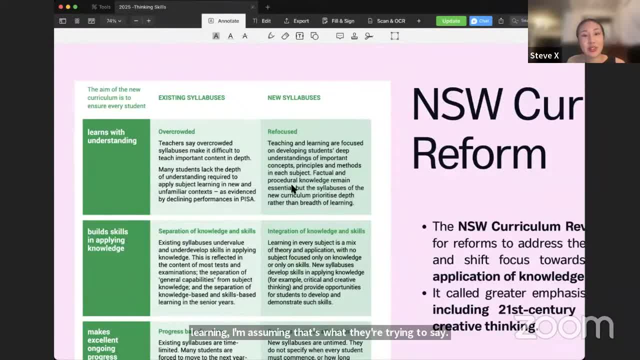 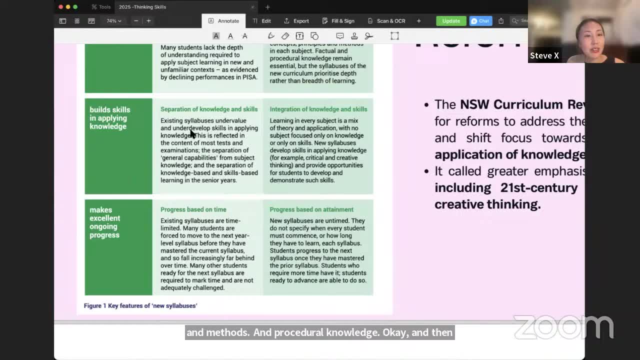 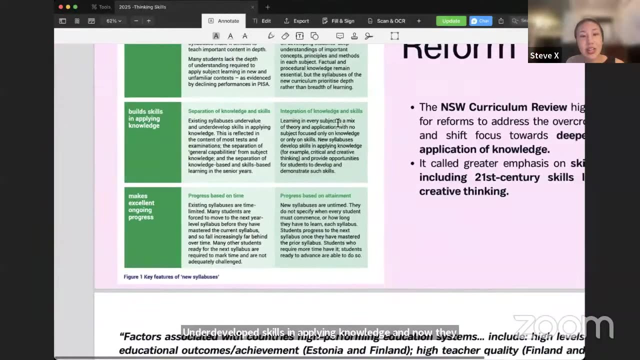 want to focus more on concepts, principles and methods and procedural knowledge. Okay, And then before they have, yeah, underdeveloped skills in applying knowledge, and now they want to apply knowledge more. So I guess that's what they're trying to do And look, I'm not going. 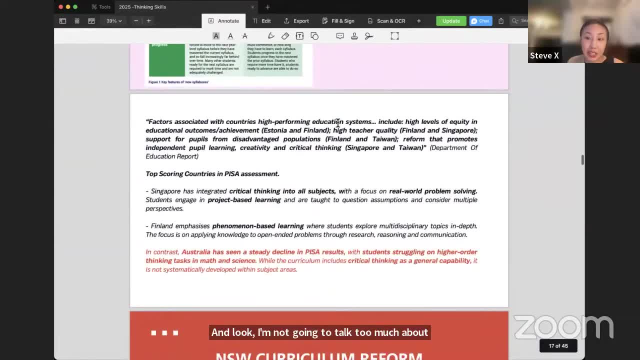 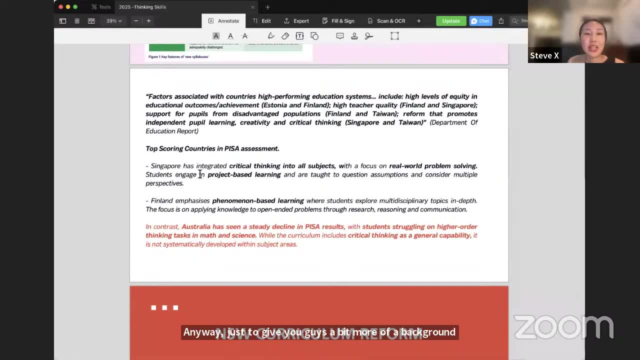 to talk too much about this. We're going to talk about how this might affect the thinking skills test. Anyway, just to give you guys a bit more of a background: other countries like Singapore and Finland and Taiwan, and like Scandinavian countries- they're so good. 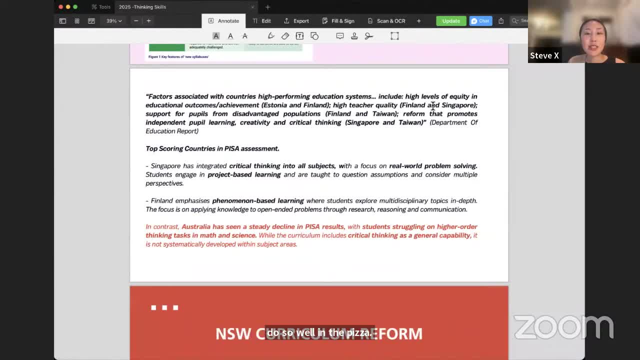 right, They do so well in the pizza, And this is from the Department of Education report. They're like: oh, all these countries right, They really focus on critical thinking and real world problem solving. So that's why they're trying to really push that in New South Wales, in Australia. 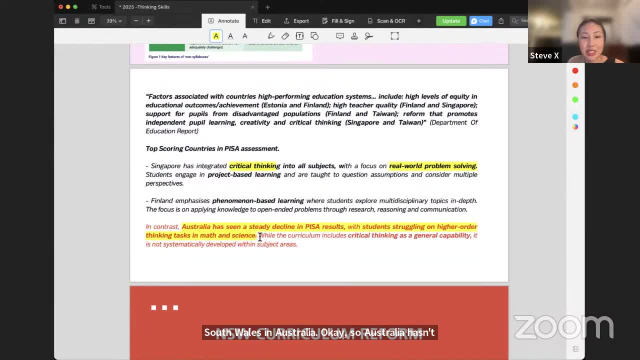 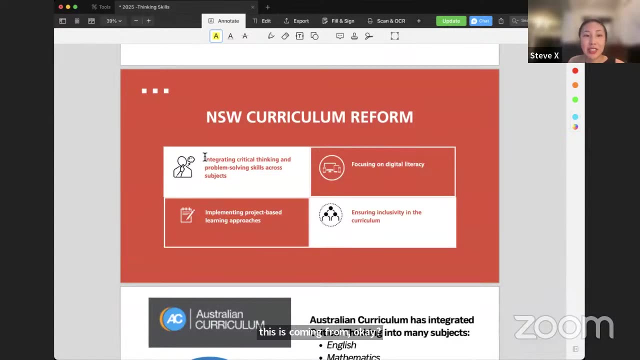 Okay So Australia hasn't done so well in pizza. unfortunately, Students are struggling with high order thinking tasks in maths and science. Okay So, this is where all this is coming from. Okay So, New South Wales curriculum reform this year. basically, they're. 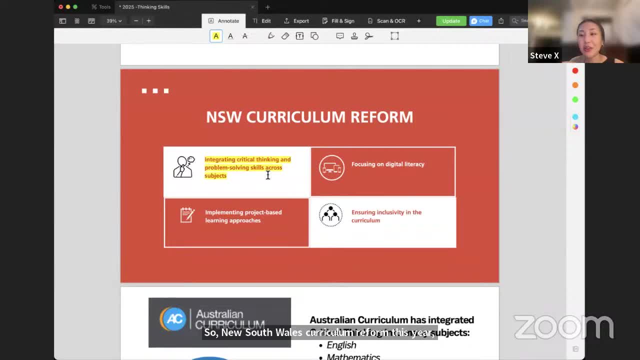 integrating critical thinking and problem solving across all subjects. You might be thinking: oh, thinking skills is just like the school thing. No, you're going to be happy, You have to deal with that until high school, right, Unfortunately? Well, fortunately. but if you're tired of hearing, 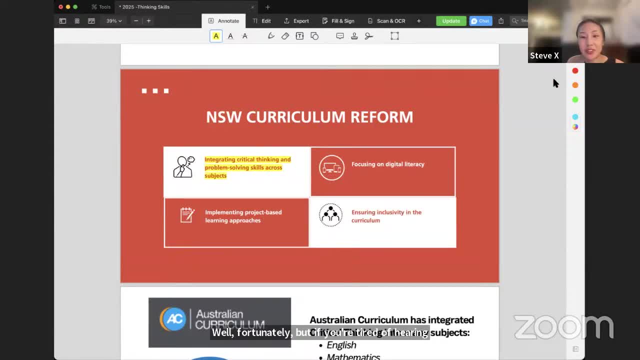 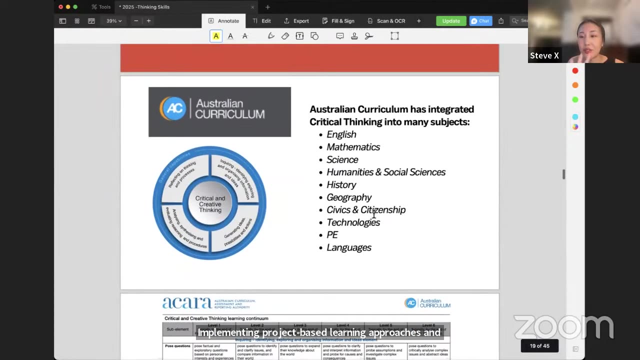 thinking skills. well, this is not the end of it, sadly. It will also focus a lot on digital literacy, So being able to use the internet in an effective manner, implementing project-based learning approaches and ensuring inclusivity, And then just TLDR. basically, they've integrated critical thinking into many subjects. There's like a skill. 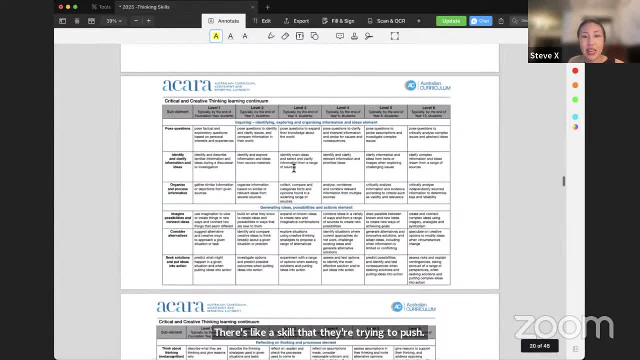 that they're trying to push. All right, So everywhere. Okay, It's just ubiquitous, no escape, And look, I'm not going to go into too much detail here, but I'm going to go into a little bit of detail here. 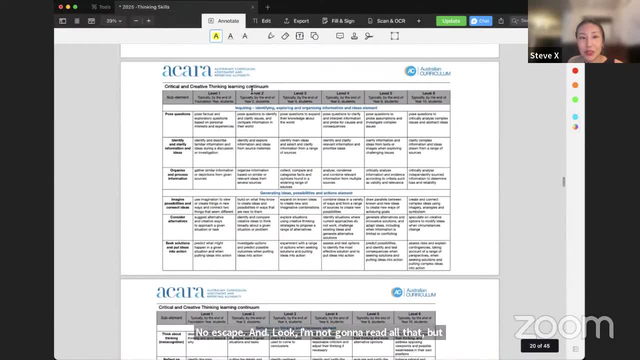 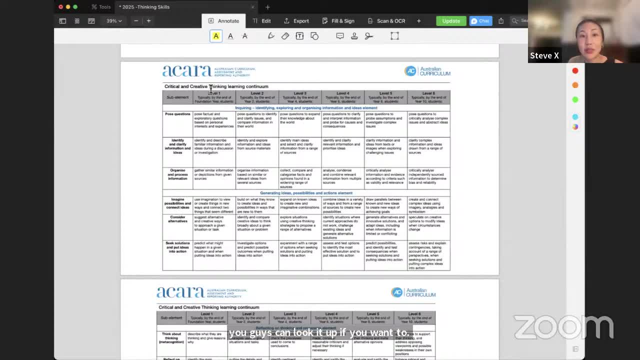 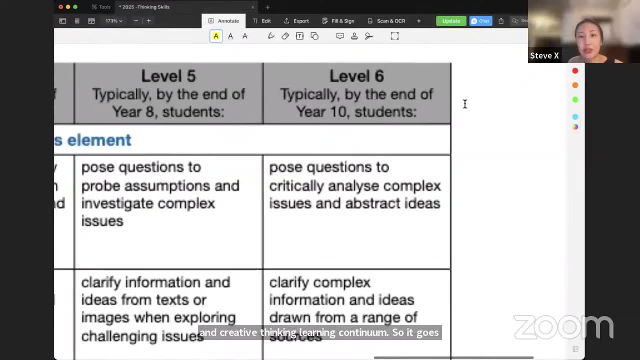 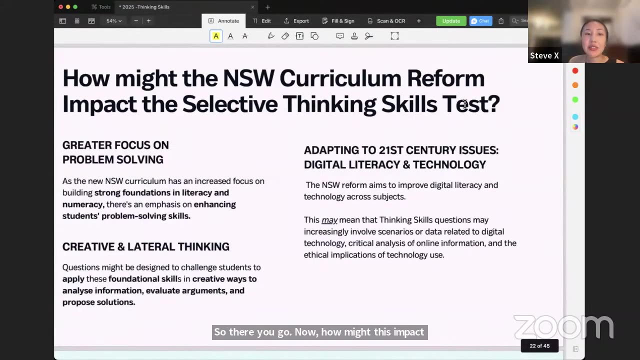 Australian Curriculum Assessment: Critical and Creative Thinking Learning Continuum. So it goes from level one, kindergarten, all the way to year 10.. So there you go. Now, how might this impact the selective thinking skills test? I think that, based on the trends and based on the fact, 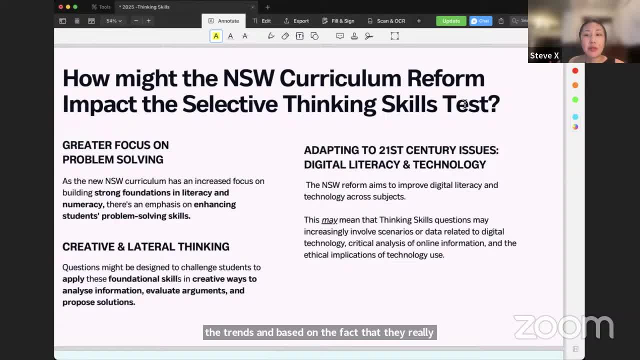 that they're really emphasising creative thinking. they will focus a lot more on problem solving questions. That's my opinion. I might be wrong to take what I say with a grain of salt, but I'm assuming that they're going to be adding in: 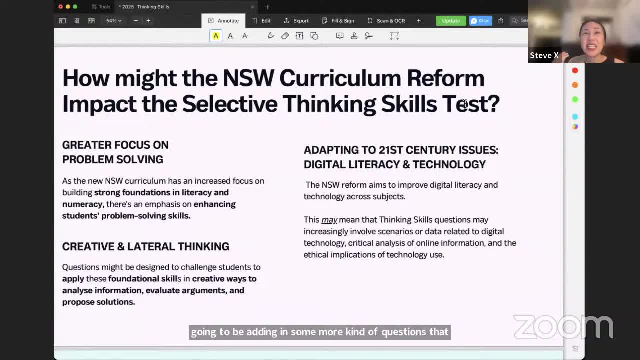 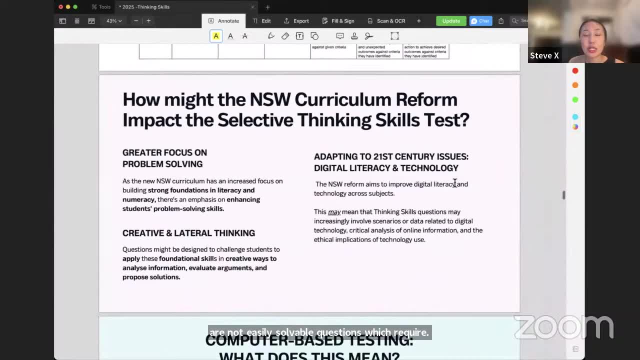 some more kind of questions that are not easily solvable, questions which require questions, which require essentially some lateral thinking, some out of the box thinking. So that is my prediction, And I think that you won't be asked to do hard maths. but 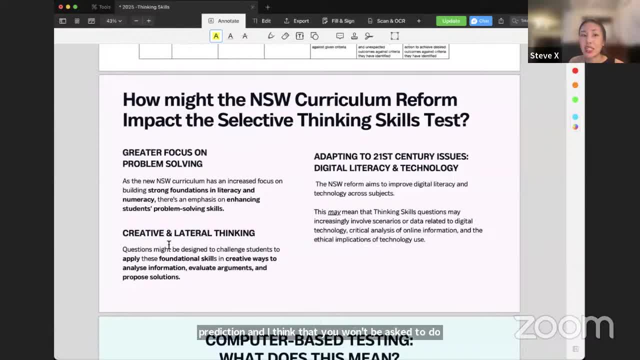 you will be asked to do questions which require a lot of experimentation and questions which require a lot of adaptability. So I think there's a real emphasis on foundational skills- the basic maths in English- but you have to be able to use those skills in order to do. 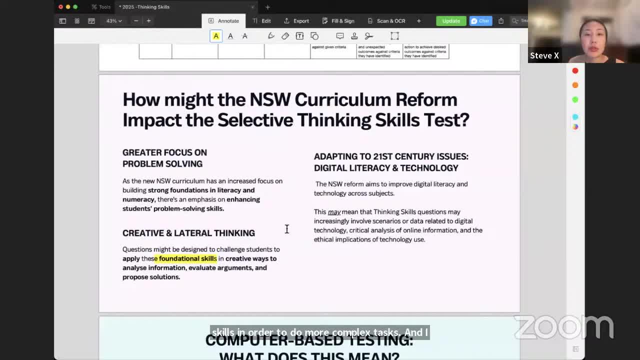 more complex tasks, And I think they might also integrate greater focus on 21st century topics, So things like digital literacy and technology, So maybe even like critical analysis of online information, because they're all about the 21st century changes, right? So those are possible predictions. 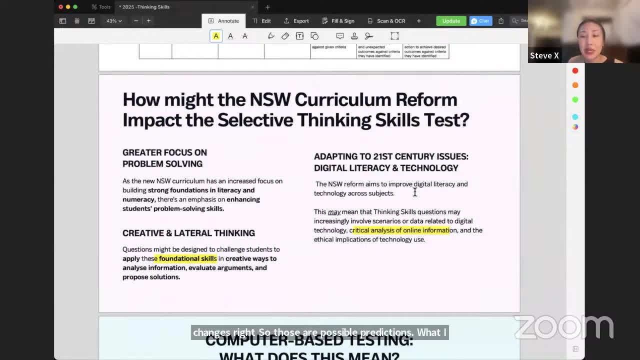 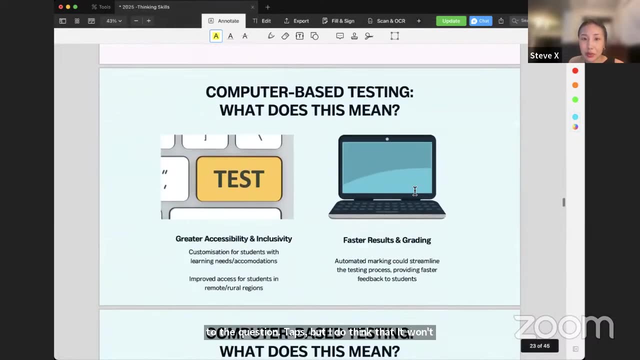 What I can say from this kind of curriculum reform is that you guys shouldn't be too stressed. I don't think there's going to be any significant changes to the question types, but I do think that it won't always be so predictable. Okay, So that's all I have to say on that. 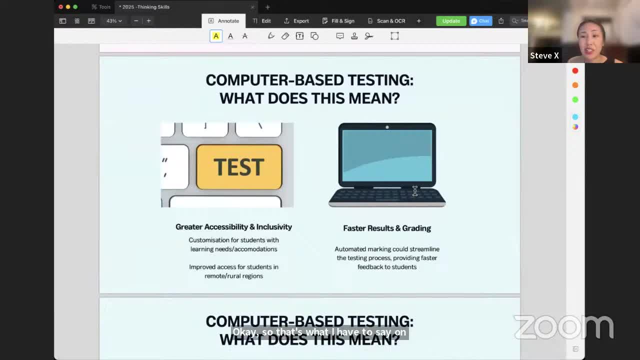 Computer-based testing In 2025.. Okay, Now let's talk about this. Why did they bring about computer-based testing? I think it's great. First of all, it increases accessibility and inclusivity. So, for students with maybe disabilities, or students who need certain accommodations- maybe they have hearing- 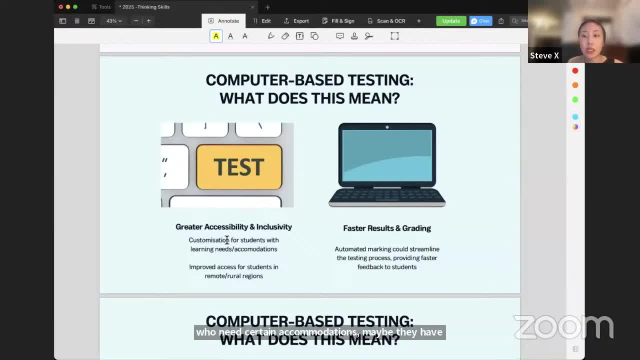 or sight problems. they can more easily sit a test Like: maybe if you're colorblind before it's very hard to do or maybe not. that's not the best example, but if you have the need for certain um learning accommodations, computer-based testing is a great way to do it. So I think 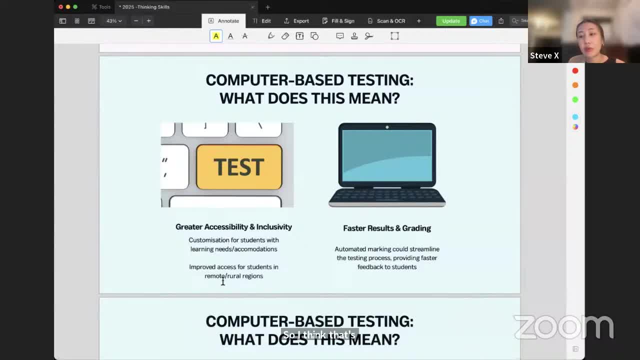 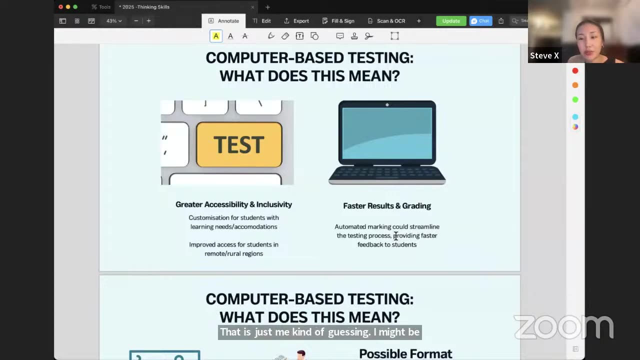 that's fantastic, And also for students who live in remote or rural regions Also. this also means that there's faster results in grading, So perhaps you'll get your marks back a bit quicker. Um, that is just me kind of guessing. I might be wrong, but if it's computer-based, they will know your. 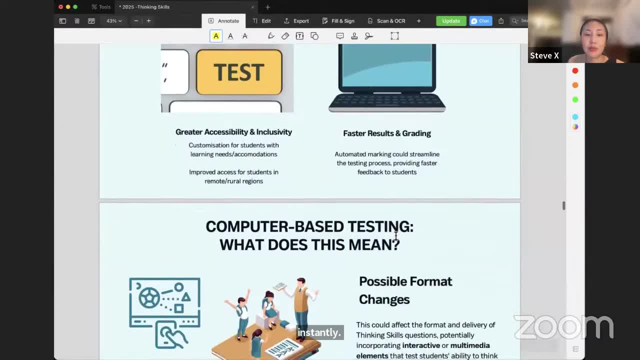 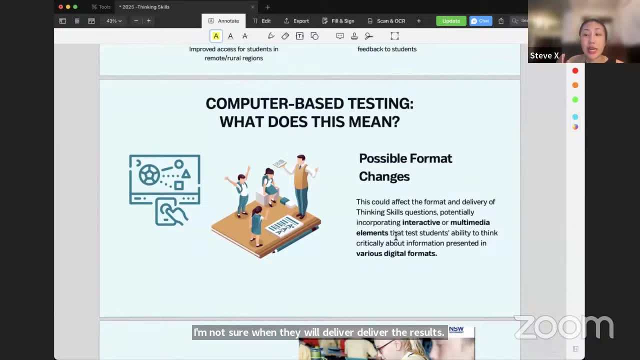 result instantly. I'm not sure when they will deliver the results, though It might also mean changes to maybe some of the media in the questions. Again, this is all tentative, but if it's computer-based they might incorporate more interactive or multimedia elements. Okay, 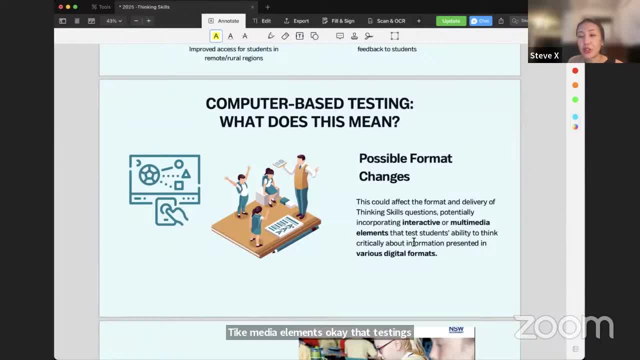 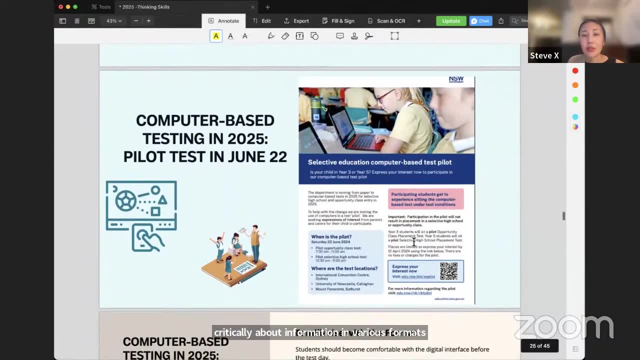 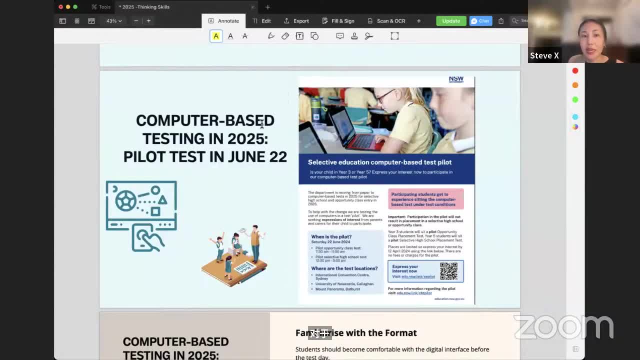 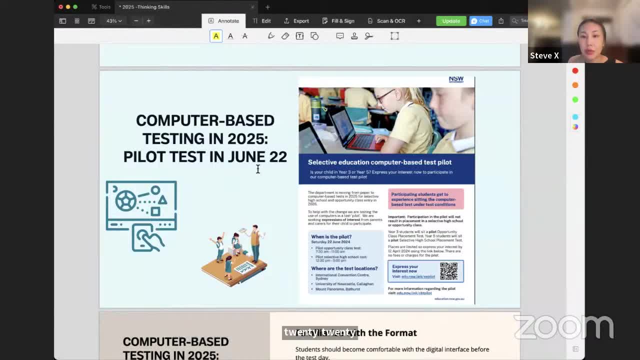 you guys have heard of the pilot test, but essentially some students will be invited to sit the computer-based test under test conditions. So, um, there's one at the international convention center in Sydney, New Darling Harbor. Um, if you were not invited, cause I think they do it on a 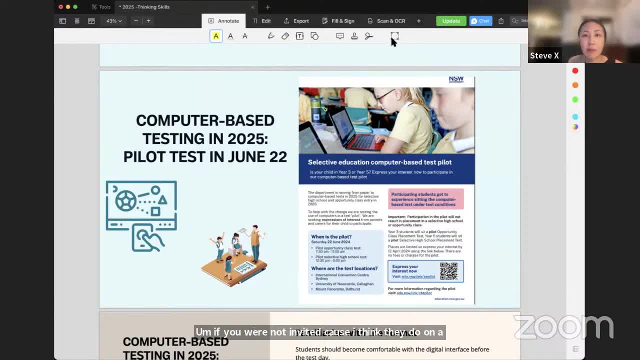 random basis. Don't stress. I think, um, we will be collating things. We will be collating things If you need feedback from our students who have gone and sat the test and we will understand exactly how it is delivered. The test itself is delivered by the same company which delivered. 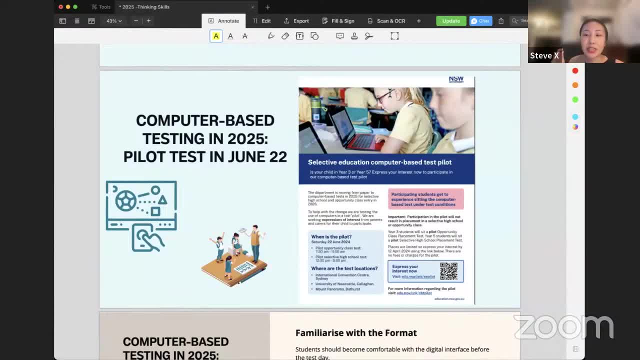 Naplan. So comment down below: have you guys done Naplan this year yet? Right, It's the same company delivering the new selective school test. Okay, And I don't know how you guys found it. Um, I don't know if you found the experience good or bad compared to when you did it in year three. 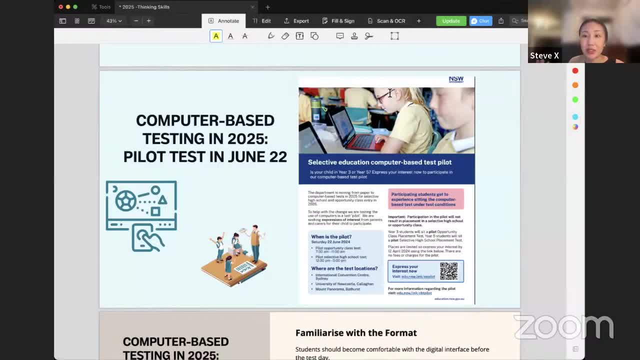 comment down below if you prefer online or like. So if you guys found your experience very positive and easy and good during NAPLAN, then you don't have to stress. okay, Nothing to stress about, because they've designed it in a way which is very easy and streamlined. 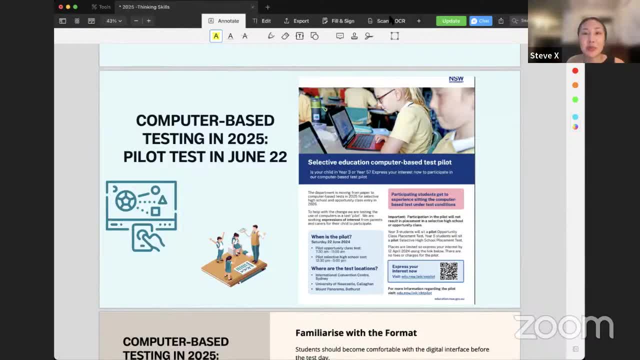 And I think it's a lot better in that when you sit a computer-based test you're not going to be making the clerical errors that you might do in a paper-based test, where maybe you'll accidentally bubble in the wrong questions. Computer-based is a bit better. 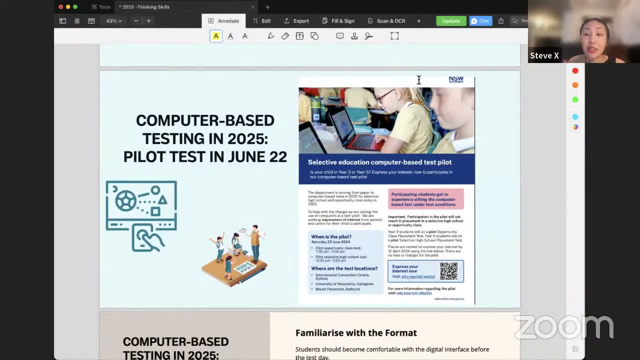 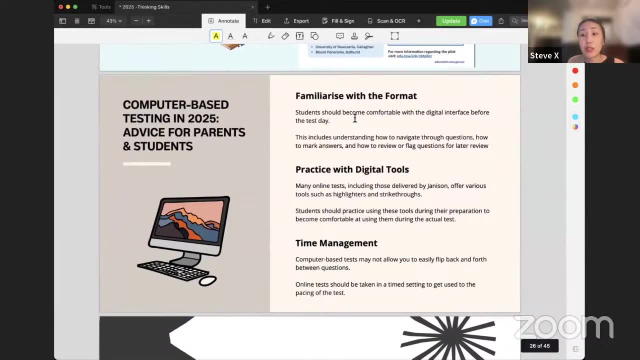 So nothing to stress about, but you do have to be familiar with the test format and you do have to have a good exam strategy. So this is my advice, I think, once we have better understanding of the exact interface and how it's delivered- 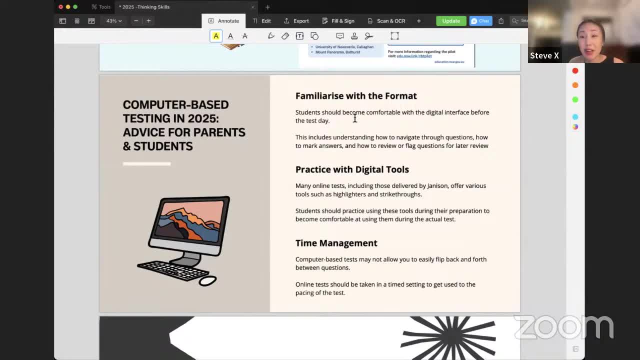 we can tell you the various tools that they might have. Maybe they have a highlighting or annotating tool. I know they did in the NAPLAN. Once we have more information then we can give you better advice. But generally speaking, try to be familiar with the format. do trial tests online right? 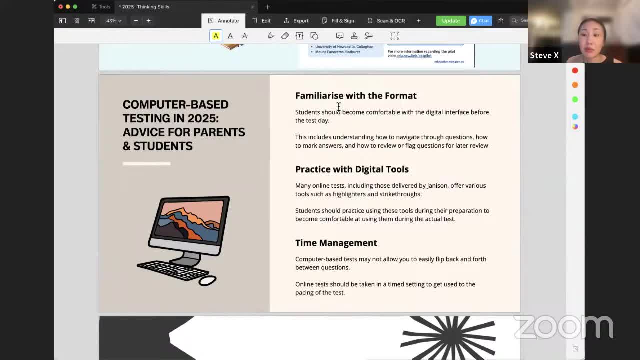 Get used to it. get used to it- Don't do a paper-based anymore because it's not going to be paper-based. and then you know, get used to navigating through the questions, knowing how to mark answers- which I know sounds silly, but you want to get used to it- and knowing how to review or flag. 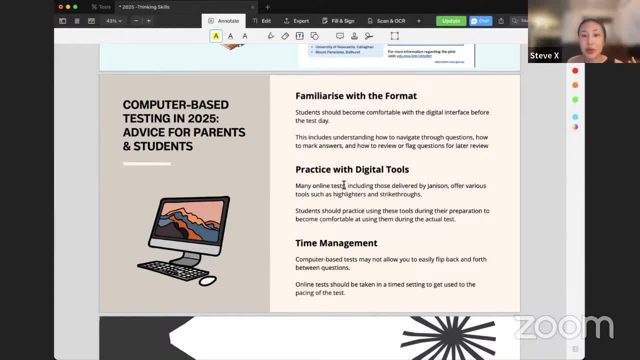 questions for later review: Practice with digital tools. So, as I've said, the test in 2025 is delivered by Jannison, which also delivered the NAPLAN test, and in the past right They've included tools such as highlighters and strikethroughs and other tools like zoom in. 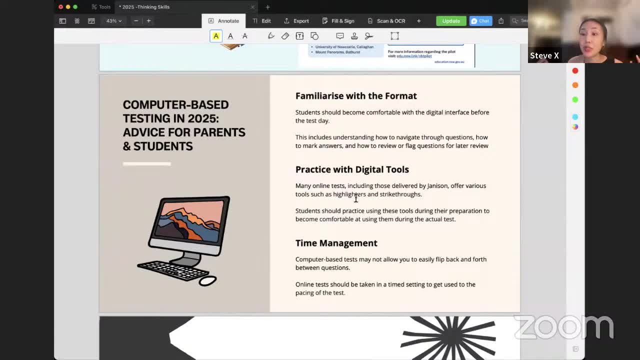 zoom out. So again, not sure how the selective score test will be, but I'm guessing it will be kind of similar and you want to be familiar with these tools during preparation. I wouldn't stress if I were you guys, because if you are scholarly you have been doing many. 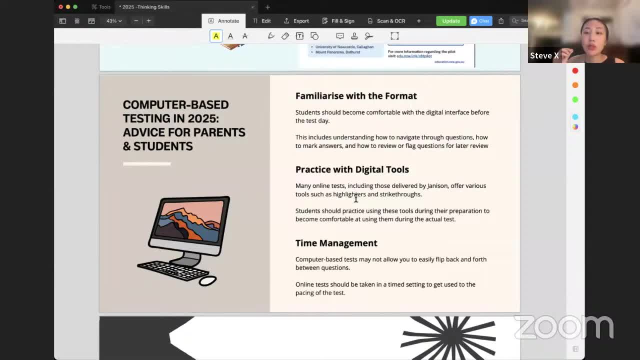 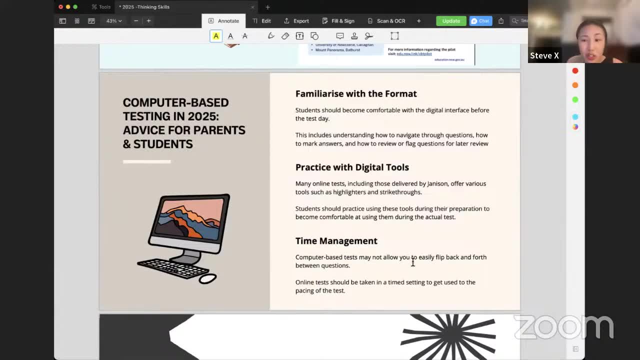 many tests online already and we will integrate all the new features onto our LMS Time management- really important. So maybe it's a little bit harder to flip back and forth between questions on a computer. So maybe make sure you have a good strategy, make sure you have, you know, comfort and familiarity. 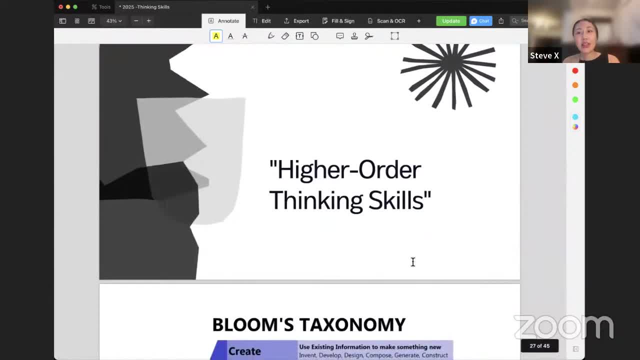 with working under timed settings. Okay, Now I'm just going to quickly talk about the secret to doing well in thinking skills and doing well in your academic journey in life. There's this thing called high order thinking skills- HOTS- Okay, It's like a buzzword used everywhere. 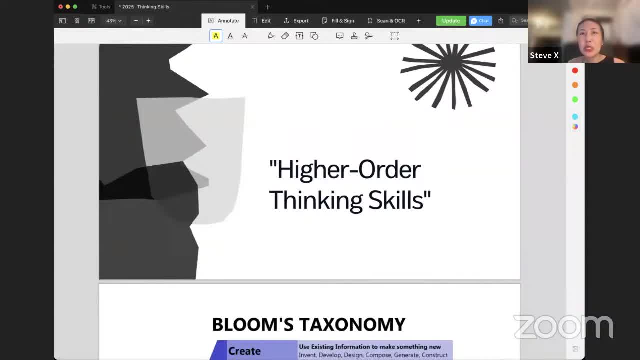 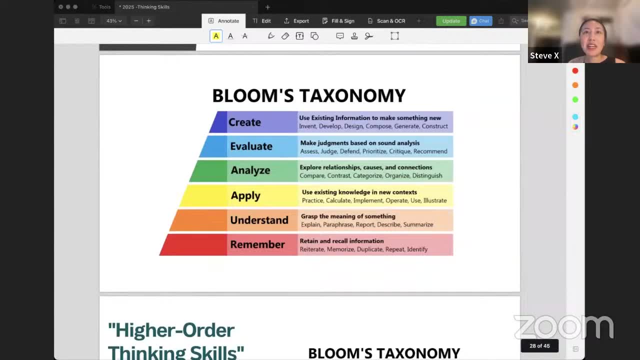 And when I first heard about high order thinking skills, I thought: what on earth is that Like? what does that even mean? So there's this thing called Bloom's taxonomy. Now, taxonomy is just a way of categorizing or ordering things, and it's organized in a 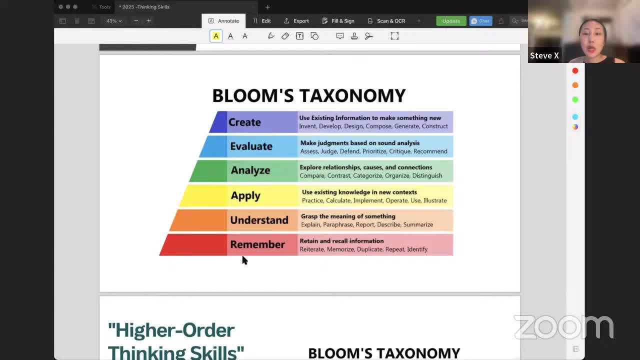 hierarchical structure, meaning it's organized from lowest to highest. So there's six categories, Okay: One, two, three, four, five, six and basically at the very bottom of this pyramid is the lowest order, uh, cognitive skill. so like, let's just say, you're learning something new, right? 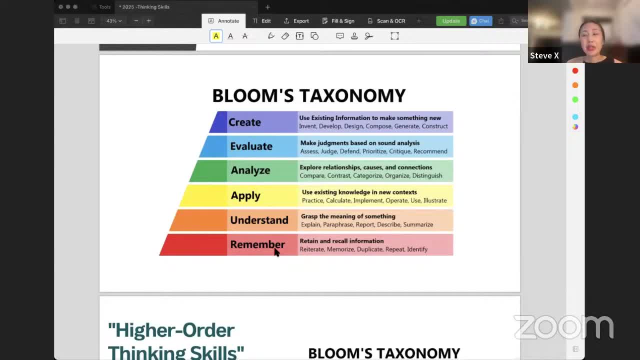 and i think about this a lot because i'm in med school and i always try to think about: hey, like i have to learn so much. how do i actually utilize this in a practical way? because i can know one niche fact, another niche fact, but if i can't use all of this together to help treat a patient, 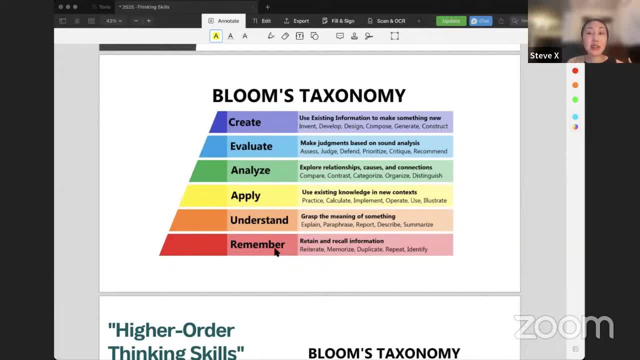 then it's kind of pointless, right? so remembering is the very bottom uh skill. so if you can just remember something like remember an isolated fact, that's a lower order thinking skill that makes any sense. the next step up is being able to understand. so grasp meaning. right, then you have to. 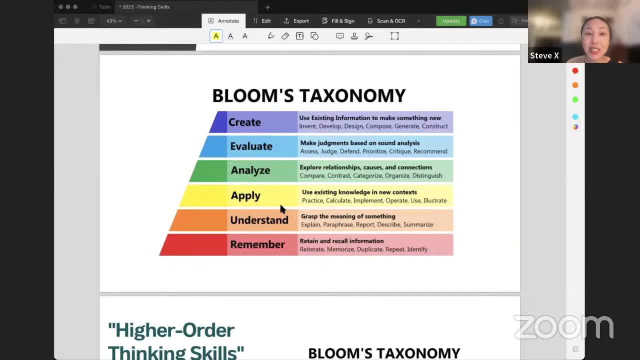 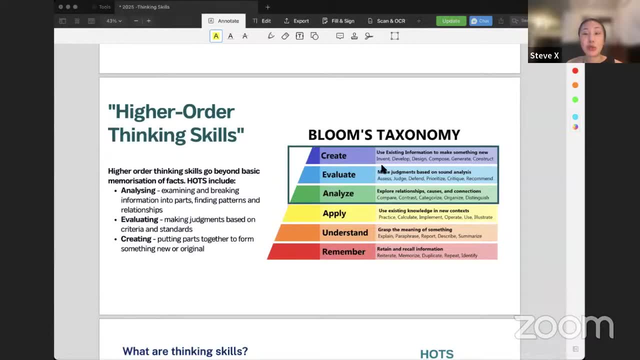 apply, so you have to be able to use that in a real world context, and then we get higher and higher. so the higher order thinking skills are basically the thinking skills at the top of bloom's taxonomy, which is analyzing, evaluating and creating. okay, and that's what they're testing. 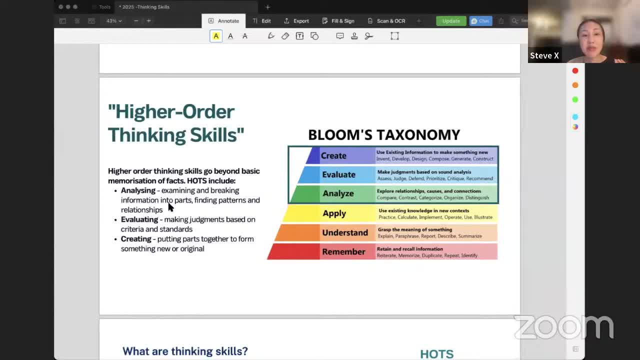 you for and that's what we're trying to do in ourorlds. so let's just say these are the i guess what we can do in our world right, so we can improve it byising the topics in which we you on in thinking skills. so analyzing is examining and breaking information into parts. 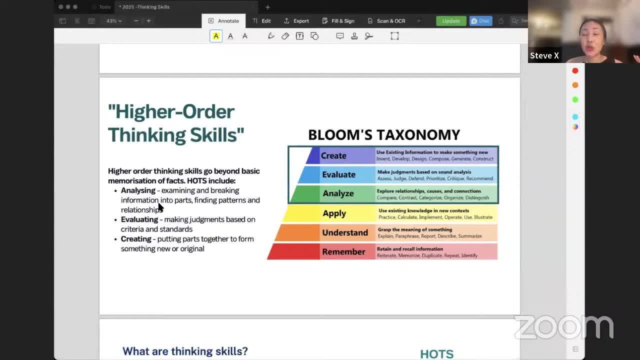 finding patterns and relationships, and that's pretty much all the problem. solving questions, right. you have so much random information presented and you have to be able to break it down into simple parts, collect the useful parts and synthesize that to come to a new conclusion or spot the patterns right, evaluating, so making a judgment, such as assessing, judging. 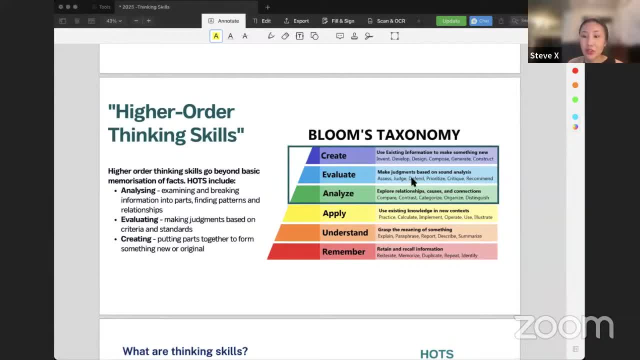 defending right. it's like when you do those strengths and weakened questions, you are assessing how strong the evidence is, you are making a judgment, you are evaluating and then, at the very top, is creating, which is use existing information to make something new. so if you are able to reach that um, like that apex, that just means that you have mastered it. you are thinking: 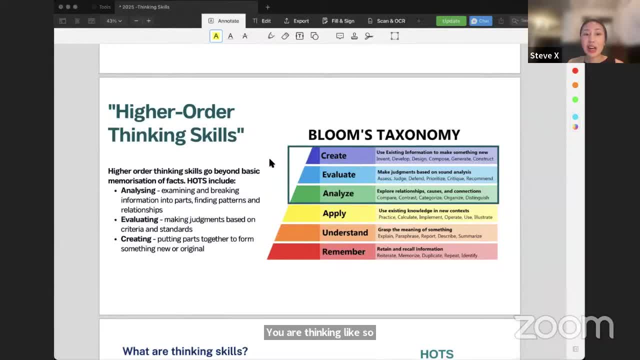 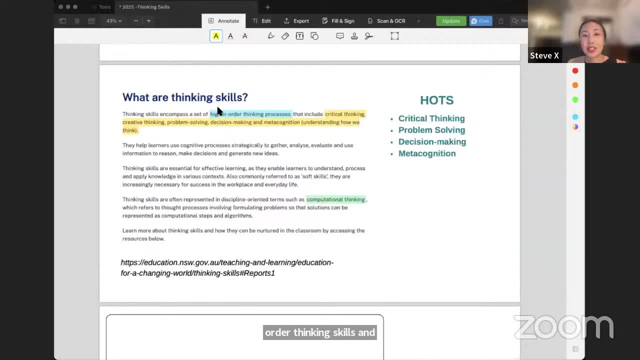 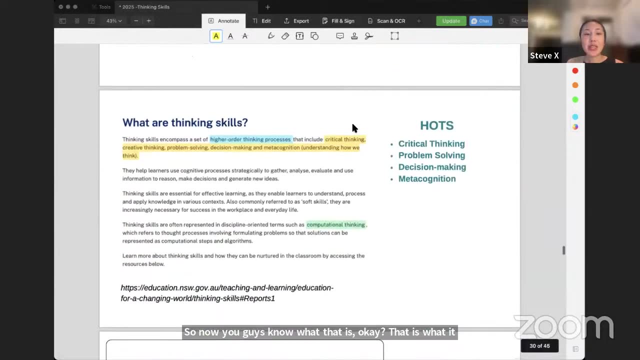 like so high right. so that is high order thinking skills, and New South Wales DLE they love the word higher order thinking skills. so now you guys know what that is. okay, that is what it is. it's just top three things in Bloom's taxonomy. now um thinking. 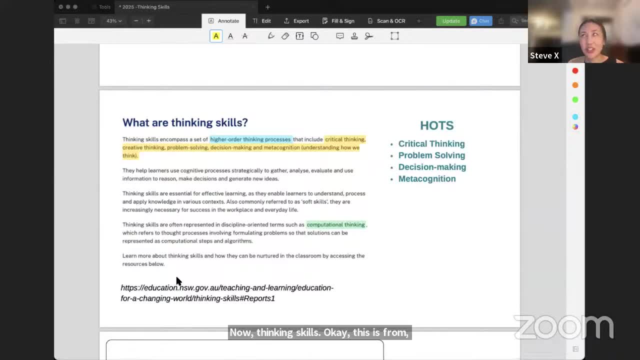 skills. okay, this is from, again, the New South Wales education website, so you can look at that if you want to. um, it's creative thinking, critical thinking, problem solving, decision making and metacognition. now we've talked about all the first two things in quite the first two things, and we're going to talk about the first two things and we're going to. 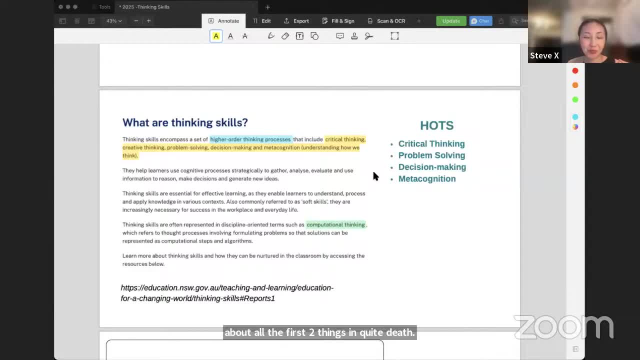 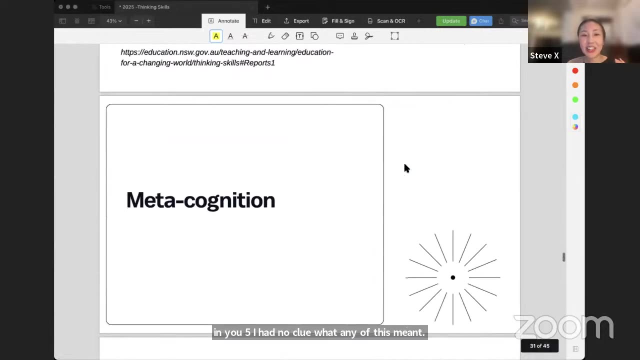 talk about death. I'm going to talk more about metacognition now. metacognition: who knows what metacognition is okay. if you don't know, don't worry, because when I was in year five, I had no clue what any of this meant. okay, so you guys are fine. metacognition is actually something really. 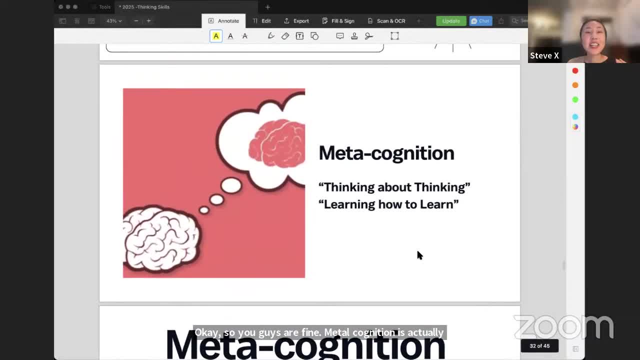 cool. okay, it is thinking about thinking, learning how to learn. okay, metacognition is when, you like, your brain is thinking about itself, which is a very cool thing to do, and I think it's actually a secret weapon to success in thinking skills. um, actually, no, it will help you much. 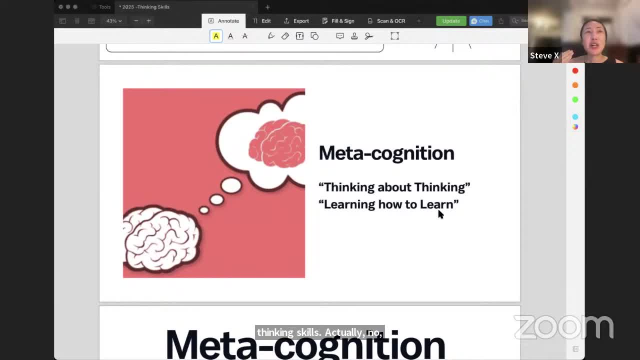 beyond just a simple multiple choice test. it will help you in high school, it will help you in university, post-grad, in life, when you start a new job and you have to learn something new. if you can apply metacognition, you're going to go very, very far. so what it is is understanding how you think. 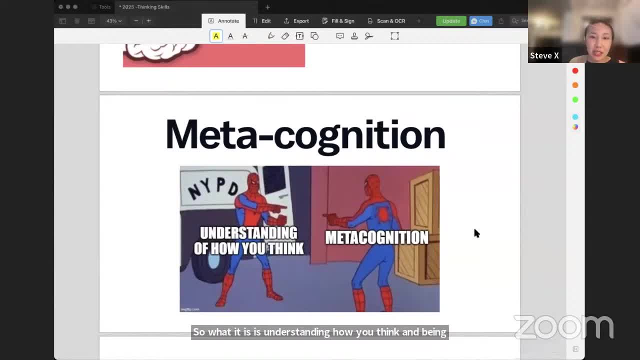 and being self-aware, and there's several things like being self-aware of your weaknesses, right, knowing where you are, um where you need further growth in right, being self-regulated, so understanding um the best way to approach something and not relying on someone else, like your parents. 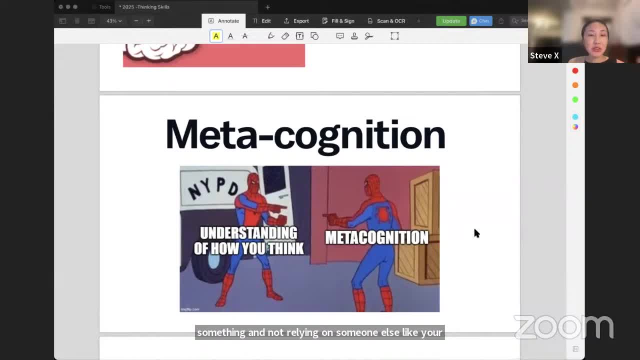 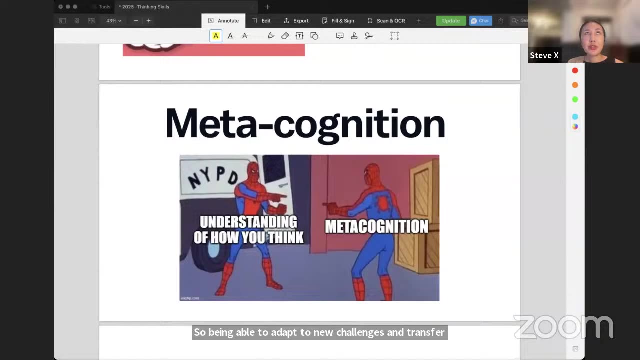 or a teacher or tutor to tell you what to do. if you can do this now in year five, you're going to go very far in life. okay, because I had no idea about any of this stuff like until I hit uni. so So, being able to adapt to new challenges and transfer your knowledge um into these different 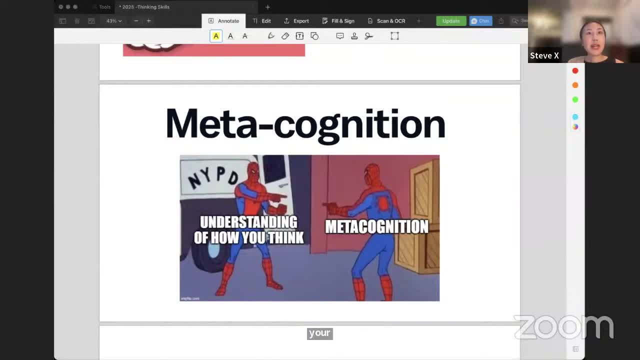 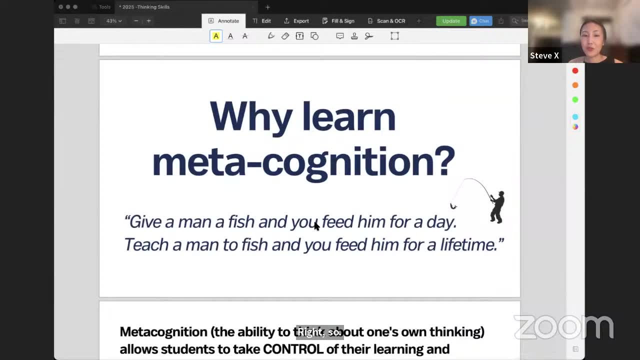 contexts. that is what metacognition is about, right? so why learn metacognition? well, when you give a man a fish, you feed him for a day. when you teach a man to fish, you feed him for a lifetime. I think that's a great quote. so what is metacognition all about? it's about learning, about learning, and 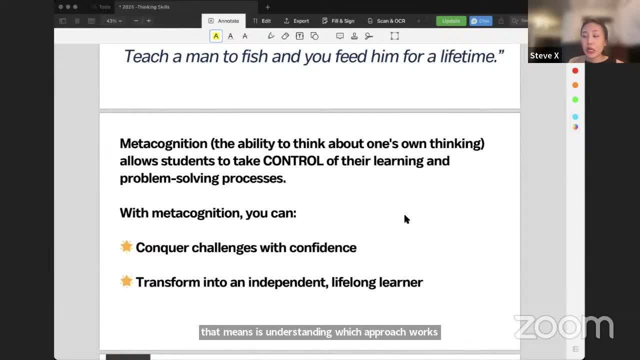 what that means is understanding which approach works best for you and what you need to do to get the best for you. understanding, um, when you do an exam, what your weaknesses are and how you can triage the questions, so know which questions to do first and which questions to flag. to come back, 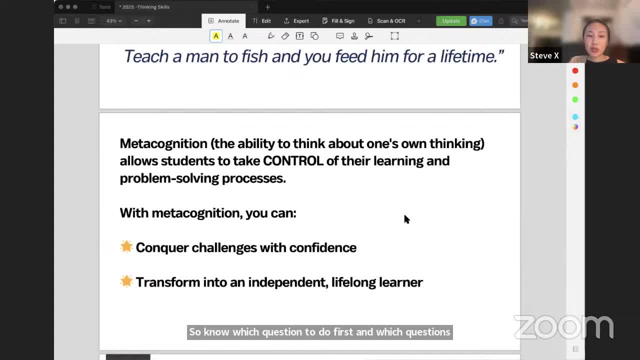 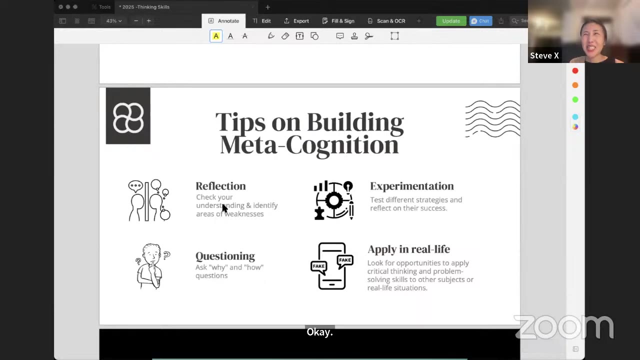 to later. um, and also try and question yourself, making errors and learning from these mistakes right, once you do this, once you make many, many mistakes and keep modifying your approach, you will understand how to do questions a lot more independently and do well, okay. so tips on building metacognition reflection. so you have to be totally honest with yourself. 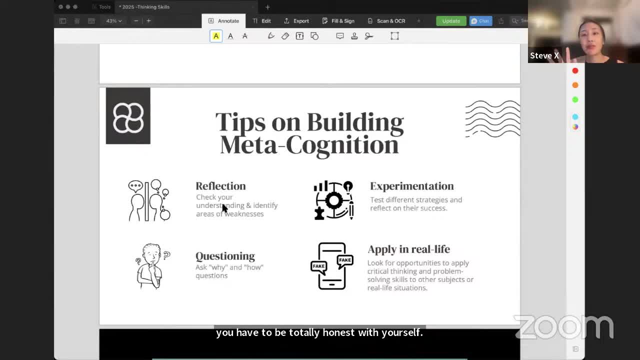 don't be delusional. don't think like I know everything because you don't. I don't know much in life. I've been very much humbled um in my medical degree so you have to realize that you don't actually know that much. and that's fine because you can learn. 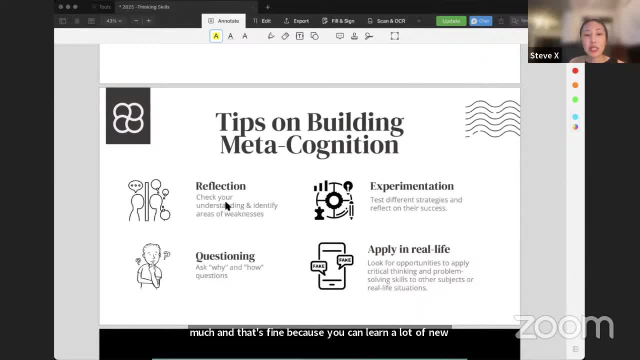 a lot of new things and learning is really, really fun. so check your understanding, identify areas of or weaknesses, experiment, so test different strategies and reflect on their success. What I've learned over many years is that what works for other people will not always work for. 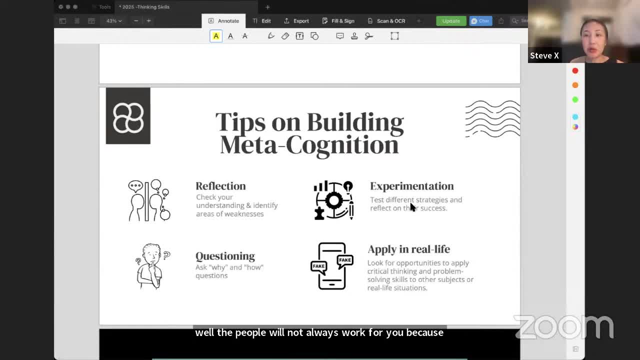 you, because everyone is different, So you have to understand yourself and you have to know which learning strategies work best for you. Another thing that will really help is questioning, So always ask why and how. If you are very inquisitive and curious, then you will start to you know. 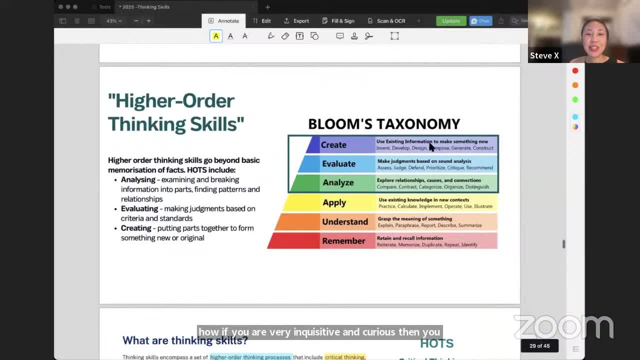 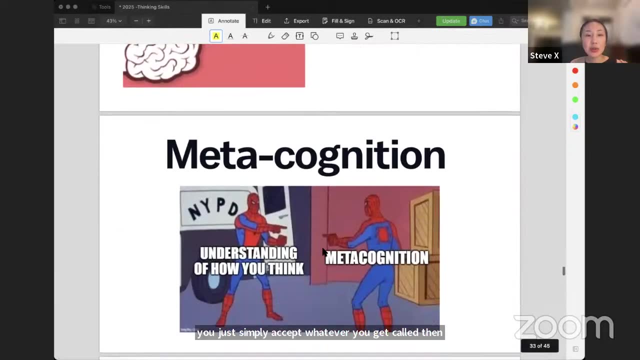 you will ascend up the pyramid and start thinking in those high order thinking skills categories. Okay, If you just simply accept whatever you get called, then you're not really going to go beyond the lower categories. So always ask questions, ask why and how and look for applications in 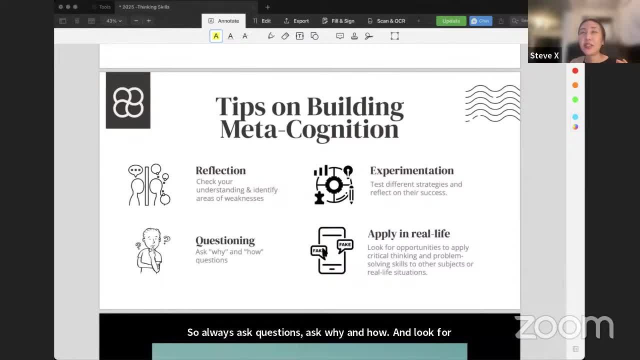 real life. Okay, Thinking skills is actually quite fun. I think it's like a fun little game that you do And you learn about a lot of concepts which you can learn about in real life. So if you're actually apply in real life, such as identifying logical fallacies and identifying questionable, 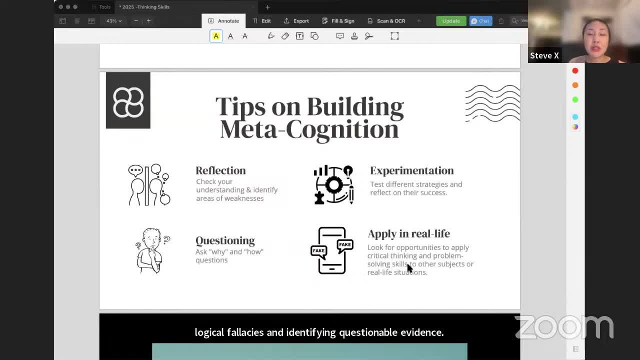 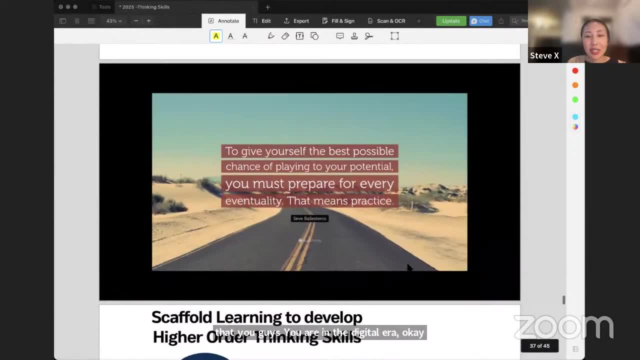 evidence. it's a very, very useful skill to have, especially given that you guys, you are in the digital era. Okay, So another thing is: you guys have a lot of time and you might think: do I have to prepare for thinking skills? Do I not have to prepare? My opinion is that you want to give. 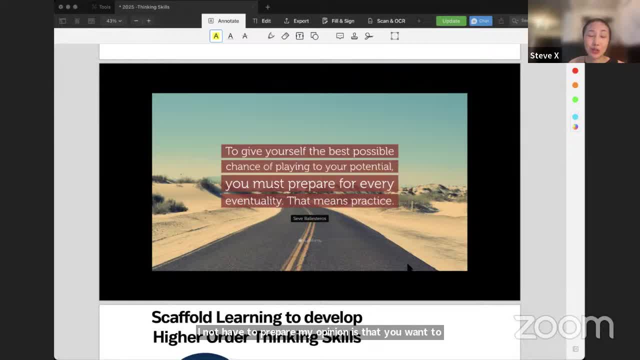 yourself the best possible chance of playing to your potential. So, to give yourself the best possible chance for success, you should try your best to prepare as much as possible. Okay, So to do that? time conditions, simulated exam conditions, creating a mistakes log book right, Reflecting on your mistakes, working out which strategy. 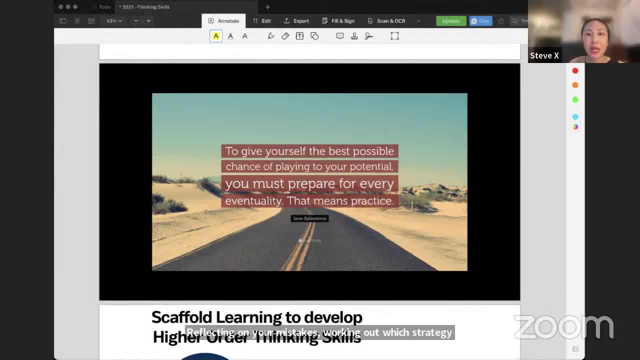 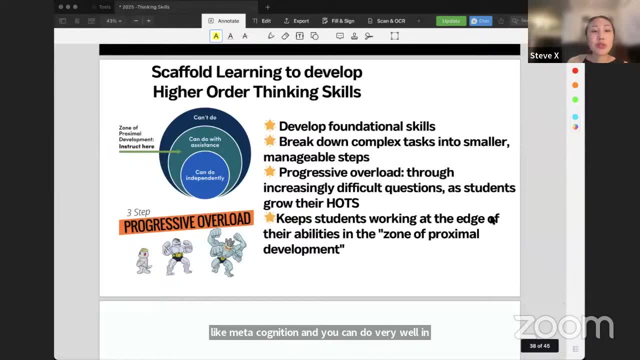 works best for you. Through that, you can apply things like metacognition and you can do very well in thinking skills. Okay, Another last thing I want to touch base on is scaffold learning. Lots of big words today, but scaffold learning is basically when you 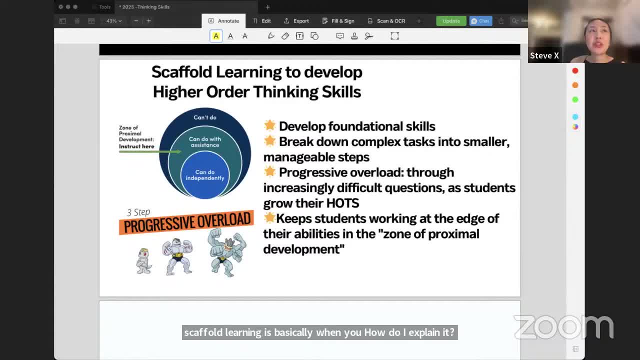 how do I explain it? It's like when you get the initial structure of how you should do something hard. Okay, So maybe a teacher like me, or maybe your parent or your sibling, your older brother, your older sister, let's just say they're teaching you thinking skills or they're teaching you math. 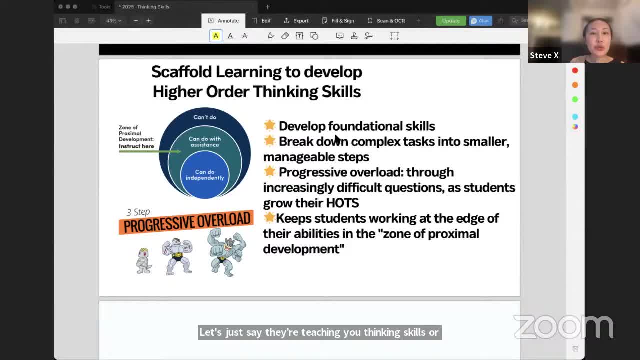 What they do is that they give you the initial foundational skills on how to do this, but then they slowly take away their support. right, So then you start doing it by yourself more, right So you're not always asking your parent or your teacher or your tutor. 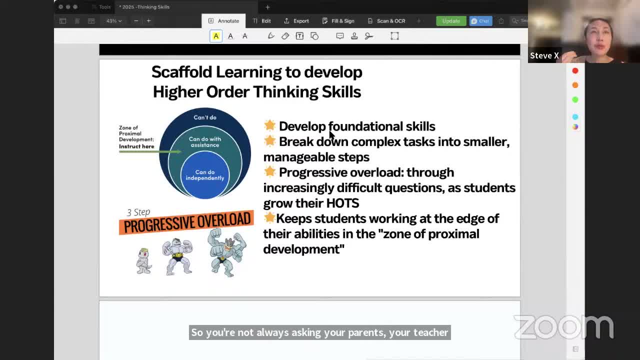 for help. And then you start trying to do more challenging and more challenging, more challenging questions until you become very, very proficient in that question type. So that is actually called the zone of proximal development. Again, that's just a very fancy word for you want to keep at. 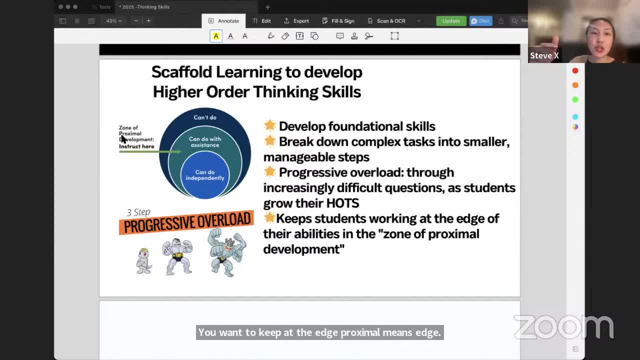 edge- Proximal means edge. You want to keep at the edge of your capabilities, So you don't always want to just be doing easy questions all day long, because then you're not, you're not going to improve. If you want to actually improve, you want to always do questions which are easy enough for. 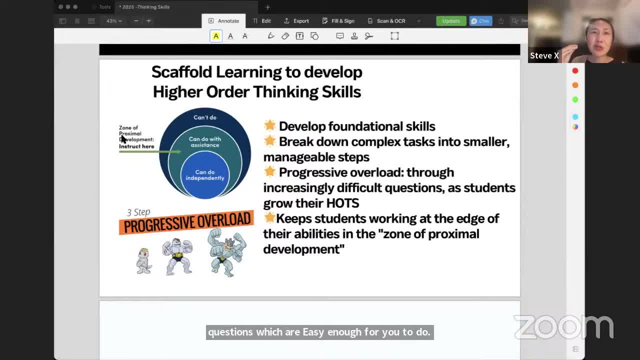 you to do, for you to understand, but still challenging enough to be at the very edge, at the very zone of proximal development in order to challenge you, for you to grow. And I think another important thing to do is make mistakes, learn. 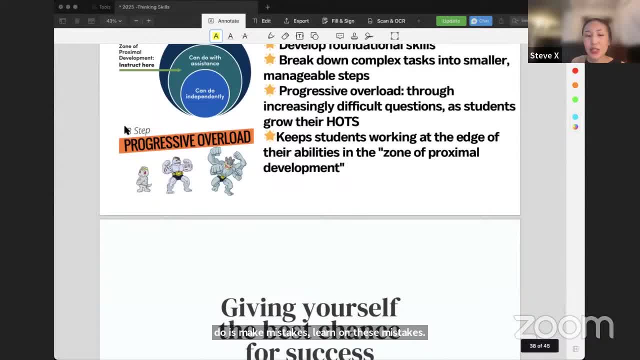 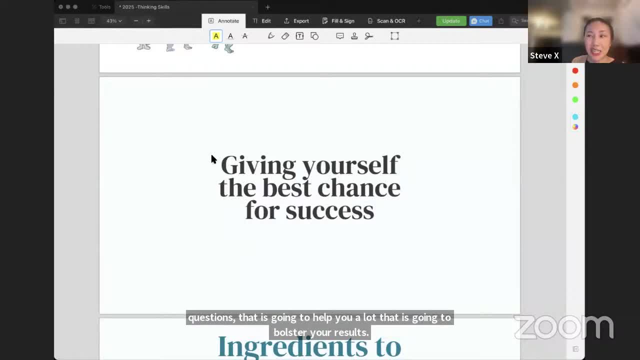 These mistakes. that way you'll do really well. So doing challenging questions, that is going to help you a lot. That is going to bolster your results. So give yourself the best chance for success. There will be people who can maybe do the test with zero preparation and ace it. 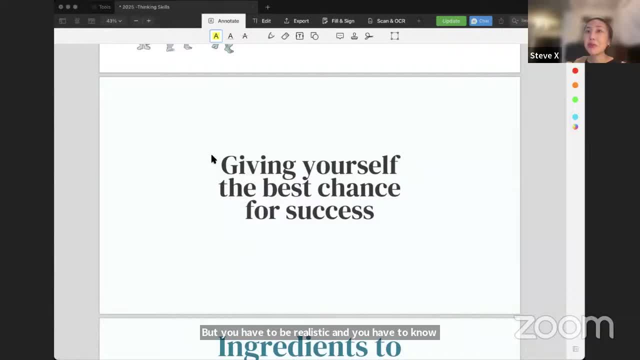 but you have to be realistic and you have to know yourself right If you are serious about getting into a top 10 selective school. comment down below. If you really want to go to a certain school, then what you have to do is go to a certain school. 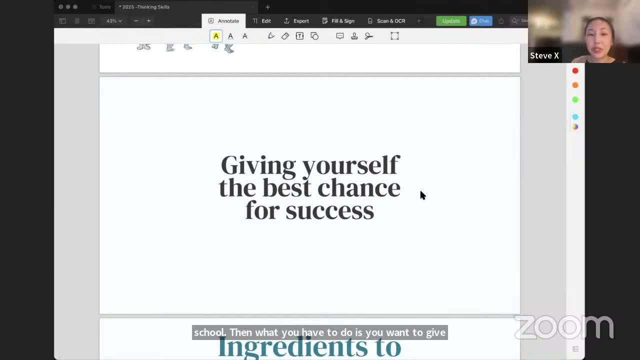 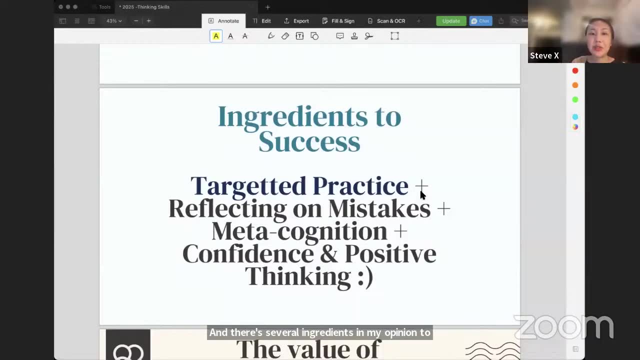 What you have to do is you want to give yourself the best chance for success, And there's several ingredients, in my opinion, to succeeding in selective school test: Targeted practice, reflecting on mistakes, metacognition, so being aware of how you're learning.